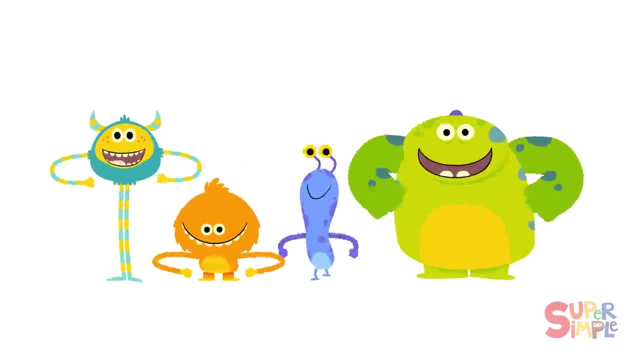 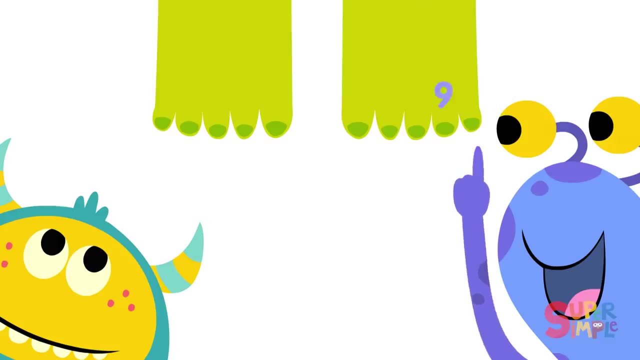 How many toes on two feet? Let's all count together: 1,, 2,, 3,, 4,, 5,, 6,, 7,, 8,, 9,, 10.. 1,, 2,, 3,, 4,, 5,, 6,, 7,, 8,, 9,, 10.. 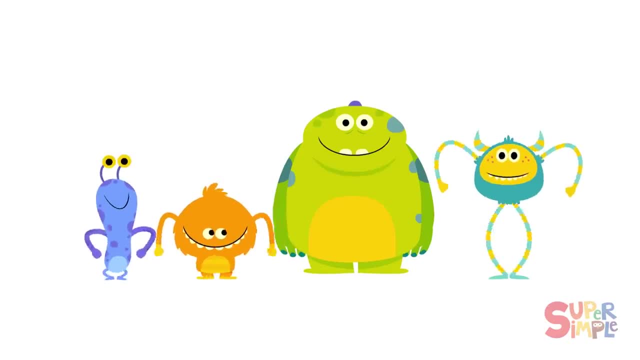 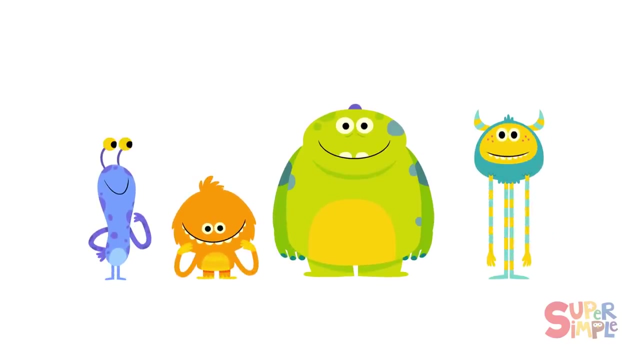 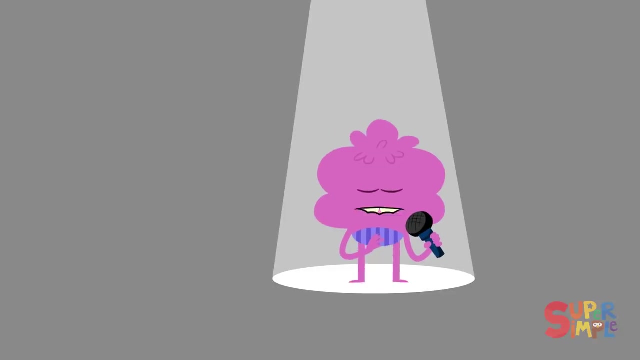 Stomp, stomp, stomp your feet, Stomp, stomp, stomp your feet, Stomp, stomp, stomp your feet, Stomp your feet with me. 1,, 2,, 3,, 4,, 5,, 6,, 7,, 8,, 9,, 10.. 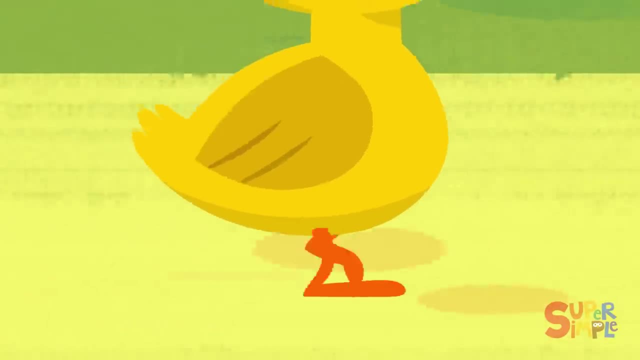 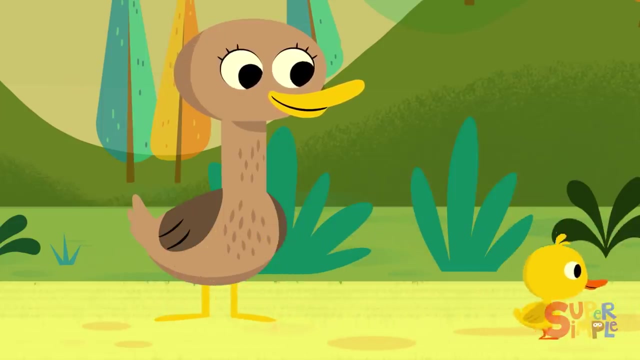 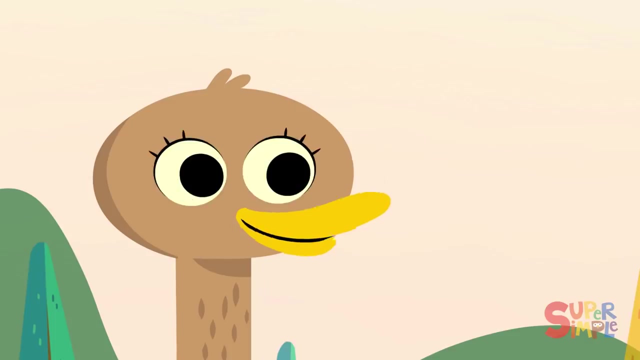 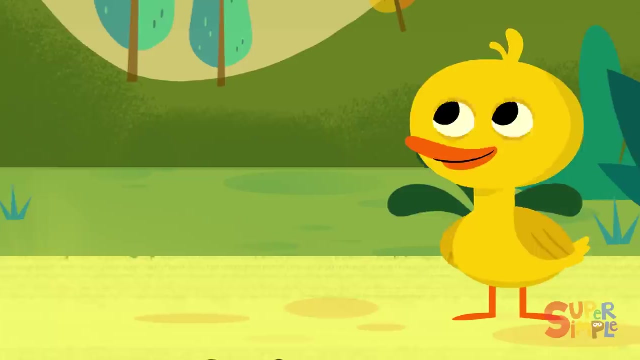 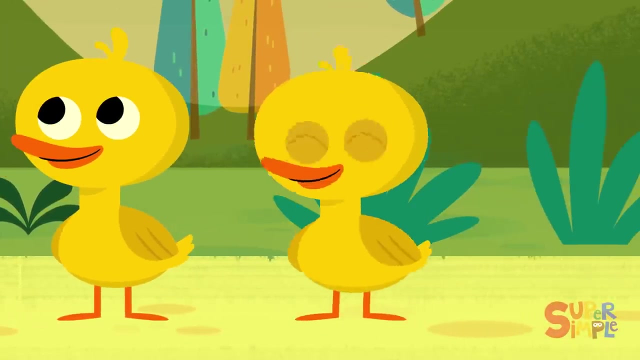 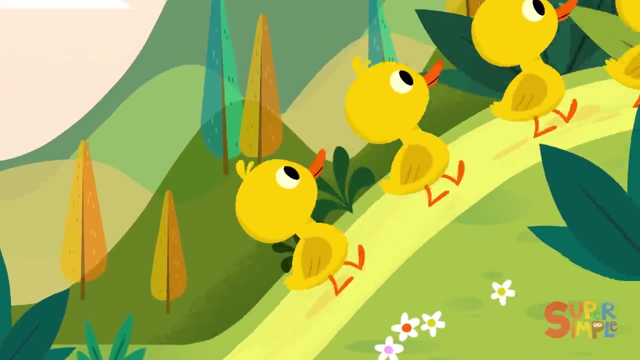 5 little ducks went out one day, over the hill and far away. Mother duck said quack quack, quack quack. but only 4 little ducks came back: 1,, 2, 3.. 4 little ducks went out one day, over the hill and far away. 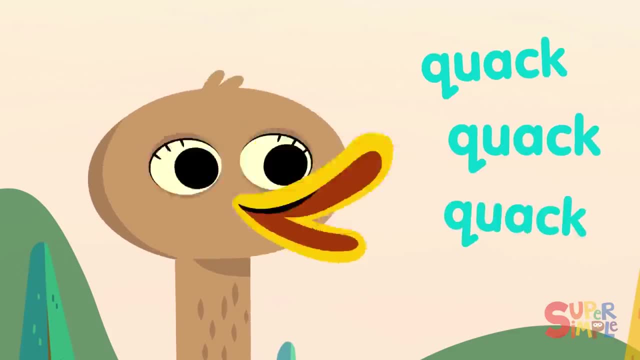 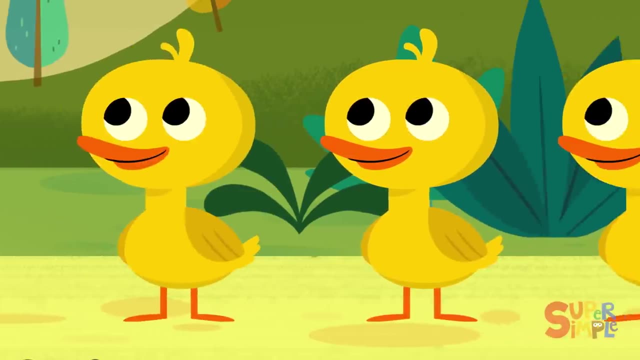 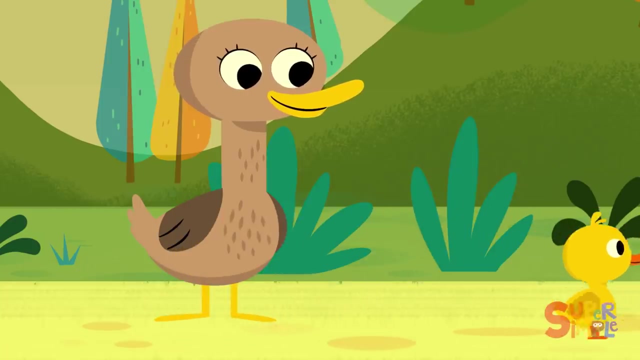 Mother duck said quack quack, quack quack, but only 3 little ducks came back: 1,, 2, 3.. 3 little ducks went out one day: 1,, 2,, 3.. 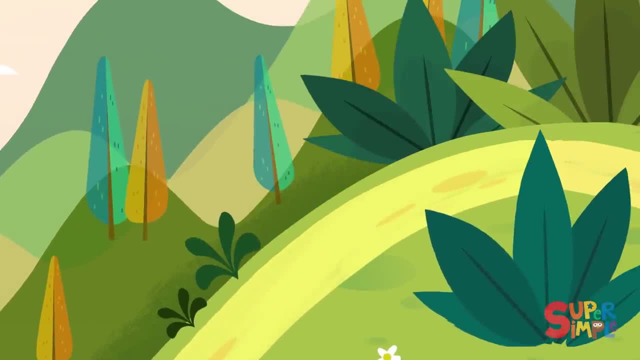 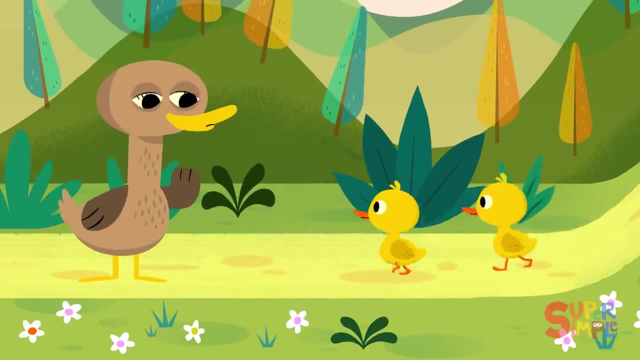 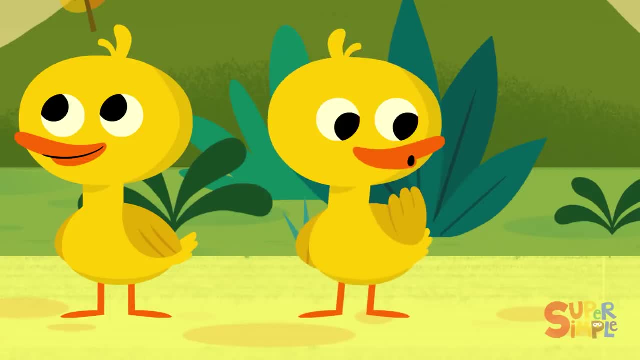 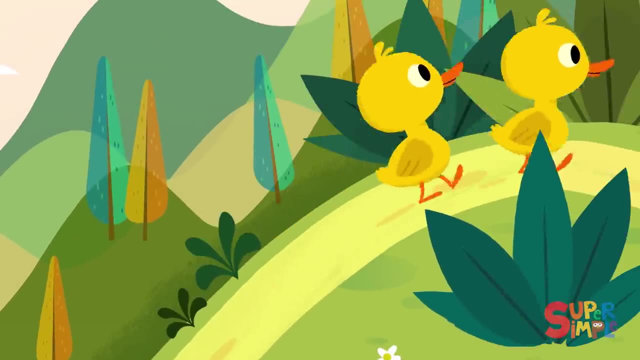 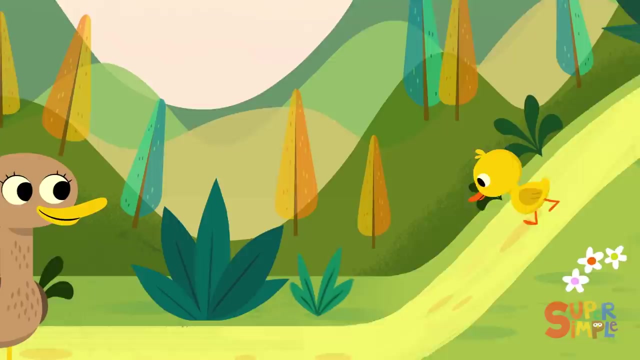 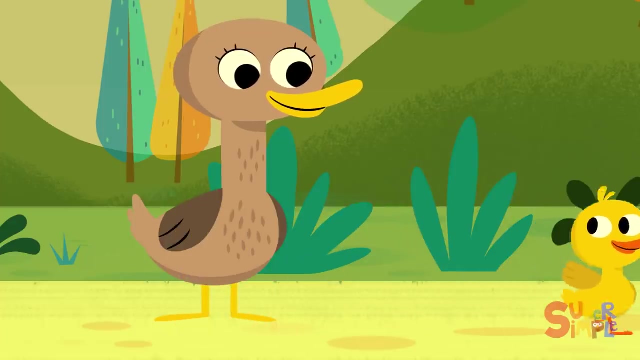 1, 2.. 2 little ducks went out one day over the hill and far away. Mother duck said quack quack, quack quack. but only 1 little duck came back. little duck came back one. one little duck went out one day over the hill and 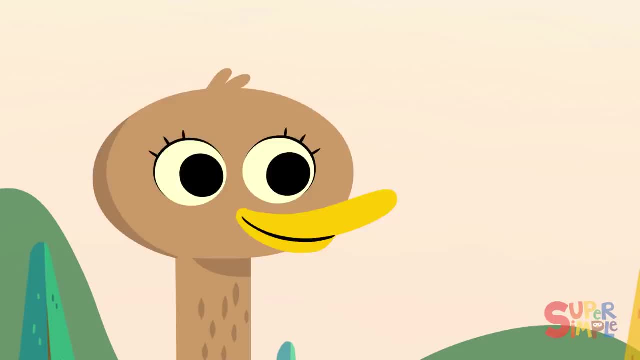 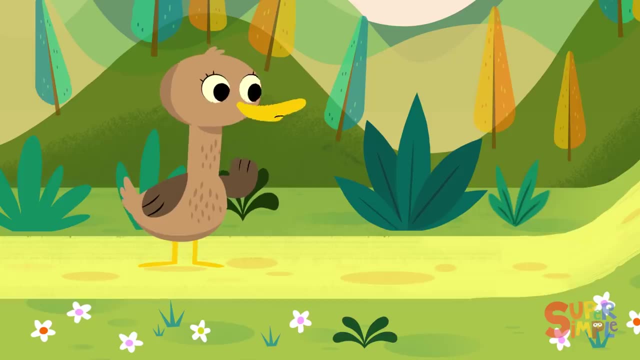 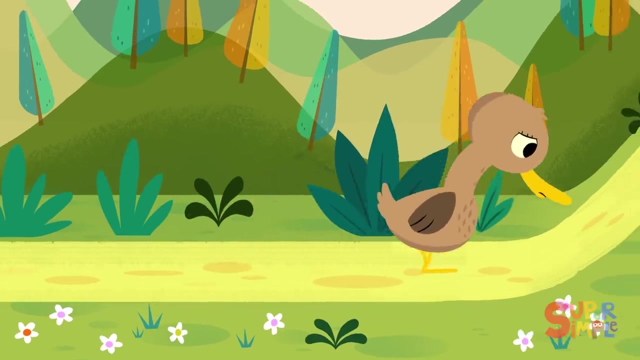 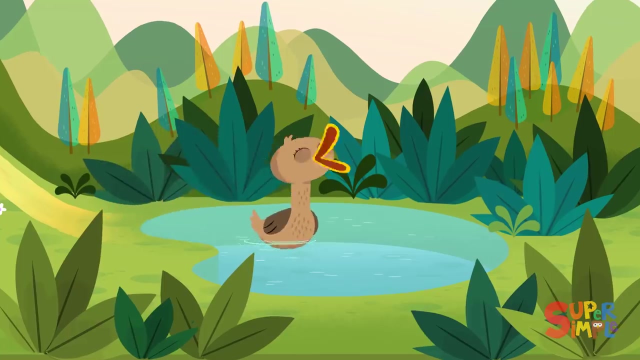 far away, mother duck said quack, quack, quack, quack, but none of the five little ducks came back. sad mother duck went out one day, over the hill and, far away, mother duck said quack, quack, quack, quack, and all of the five little ducks came. 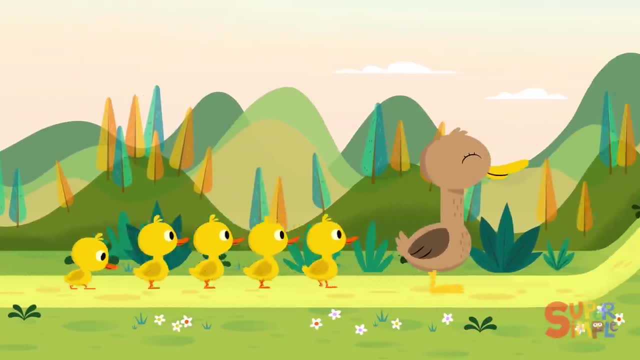 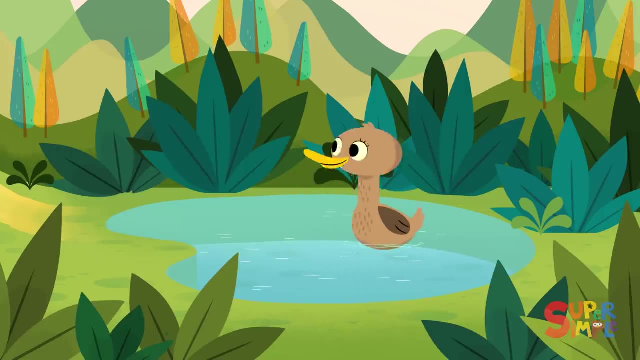 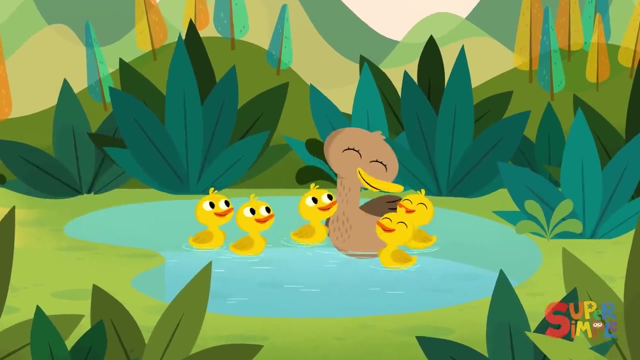 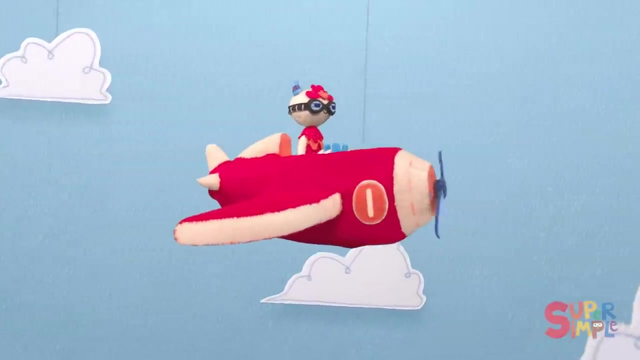 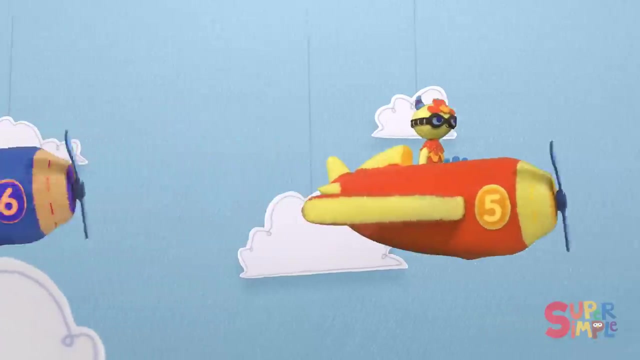 back. five little ducks went out one day, over the hill and far away, mother duck said quack quack, quack quack, and all of the five little ducks came back. let's count some airplanes: one little, two little, three little, airplanes four little, five little, six little. airplanes seven little, eight little, nine little. 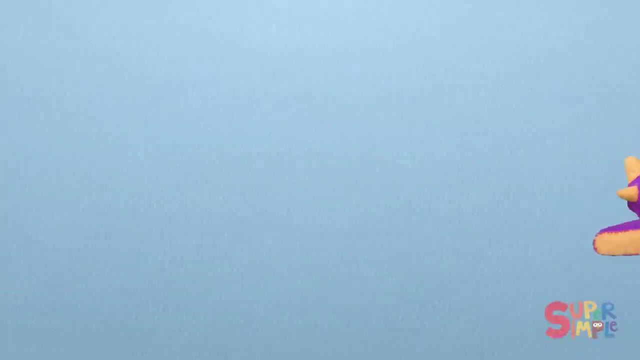 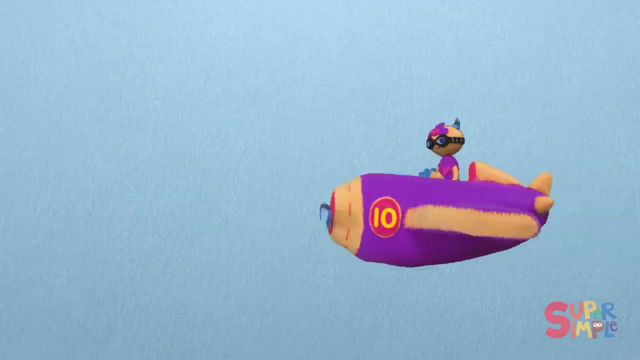 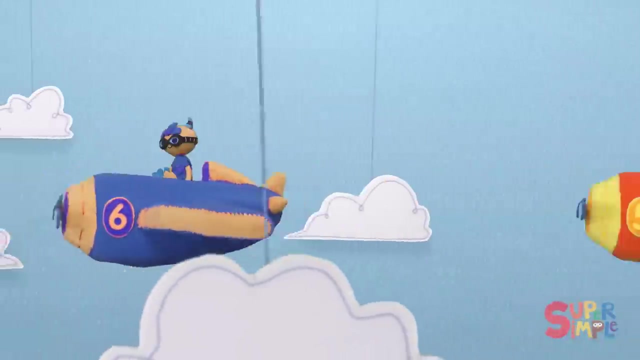 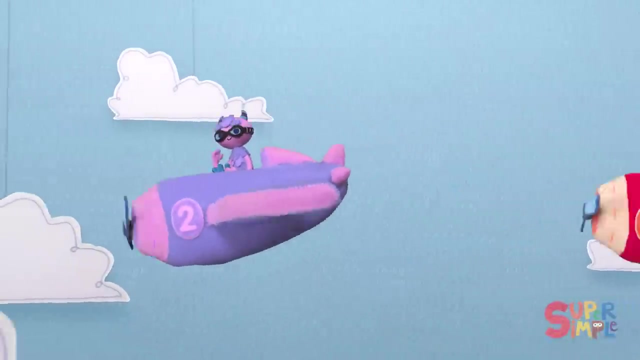 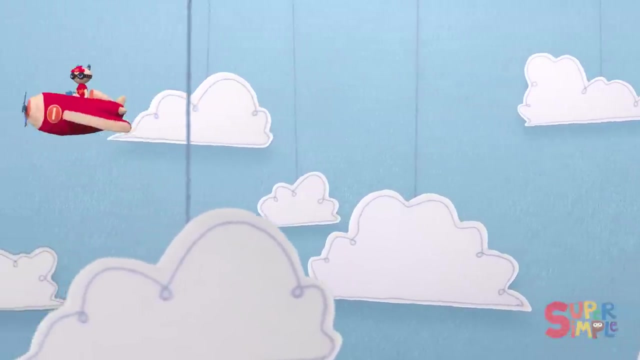 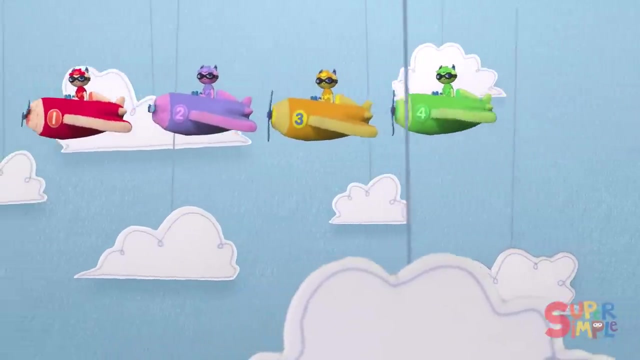 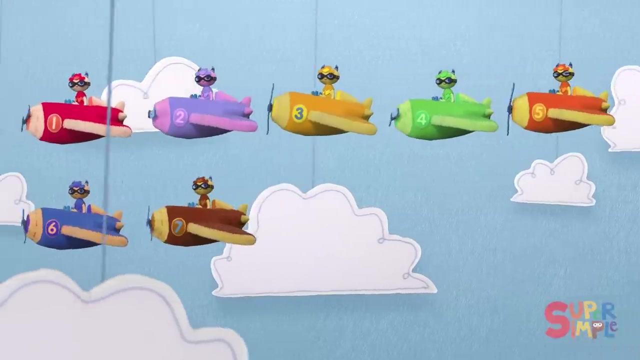 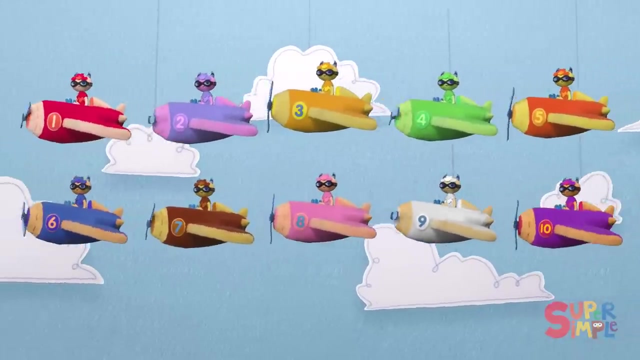 airplanes: ten little airplanes. great job, guys. now let's count backwards: ten little, nine little, eight little airplanes. seven little, six little, five little airplanes. four little, three little, two little airplanes: one little airplane. One airplane, two airplanes, three airplanes, four airplanes, five airplanes: six airplanes, seven airplanes, eight airplanes, nine airplanes, ten airplanes. 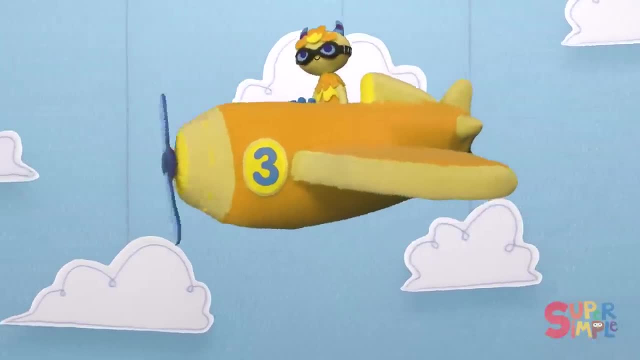 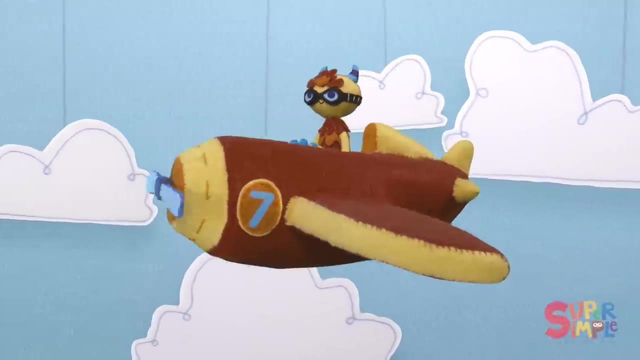 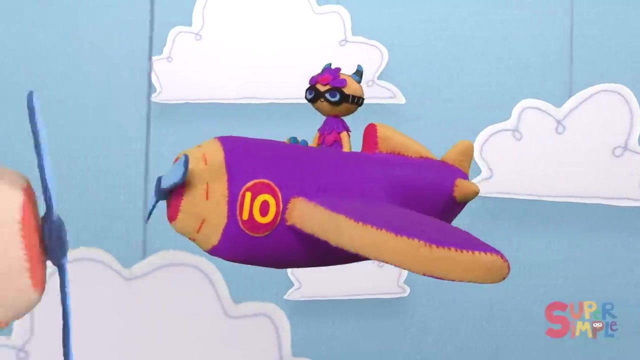 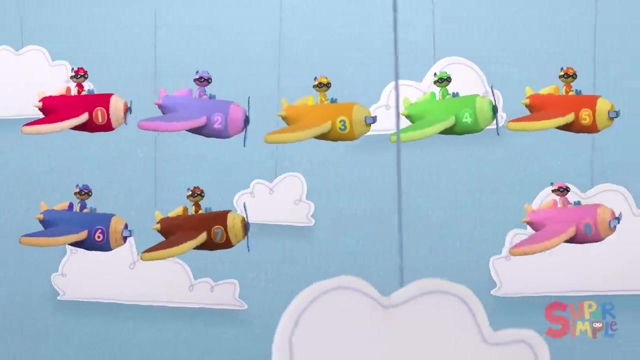 One little, two little, three little airplanes. four little, five little, six little airplanes. seven little, eight little, nine little airplanes. ten little airplanes: Ten little, nine little, eight little airplanes. seven little, six little, five little airplanes. 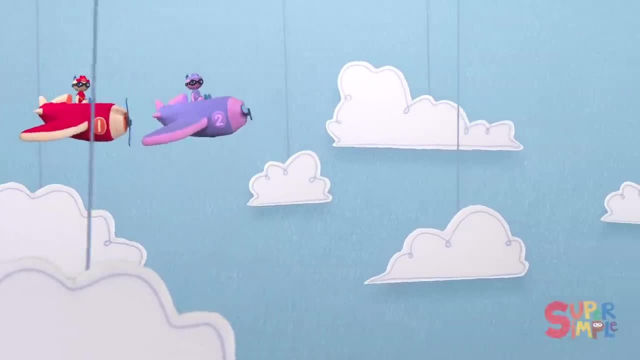 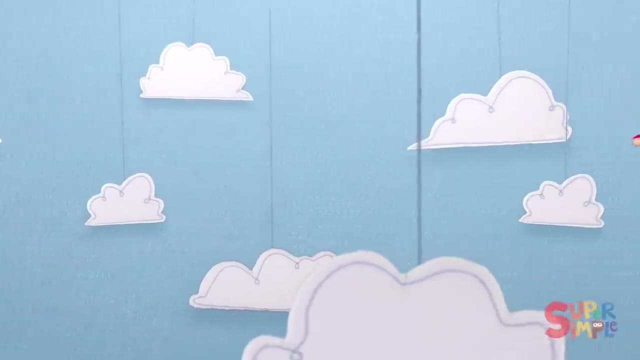 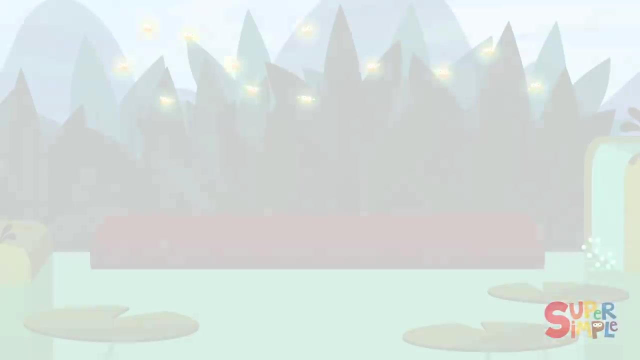 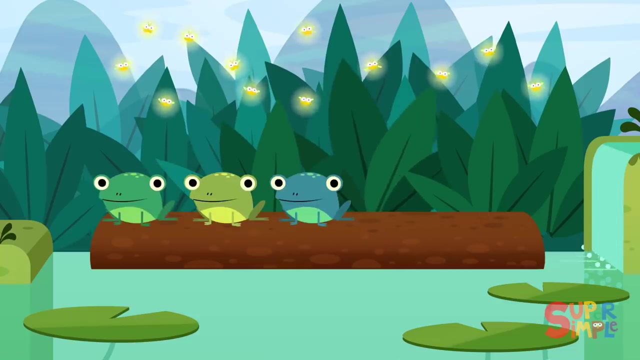 Airplanes: four little, three little. two little airplanes: one little airplane. That was fun. Thanks for counting with me. Five little speckled frogs sat on a speckled log eating some most delicious bugs. Yum, yum. 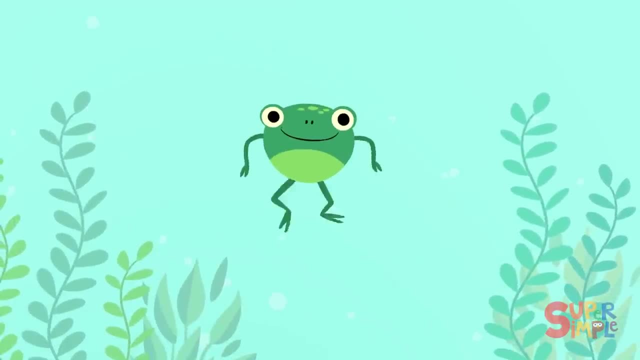 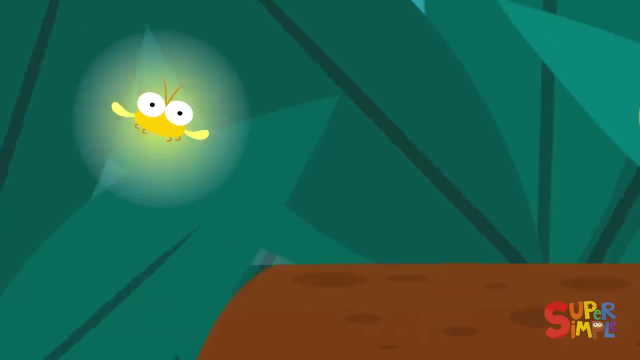 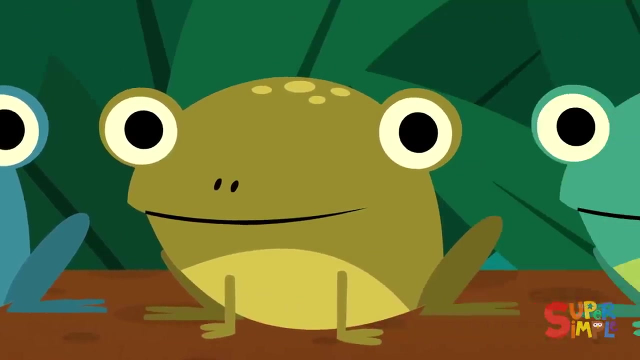 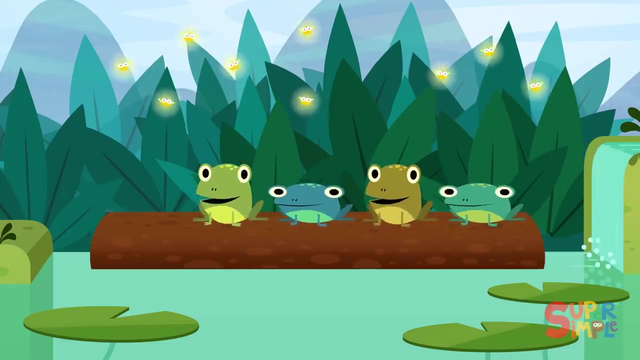 One jumped into the pool, where it was nice and cool. Now there are four green speckled frogs, Glub glub. Four little speckled frogs sat on a speckled log eating some most delicious bugs. Yum, yum. 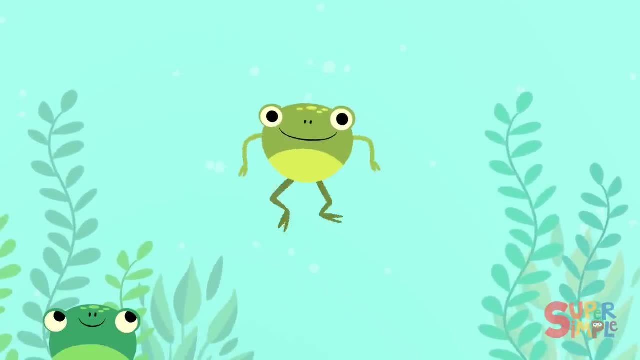 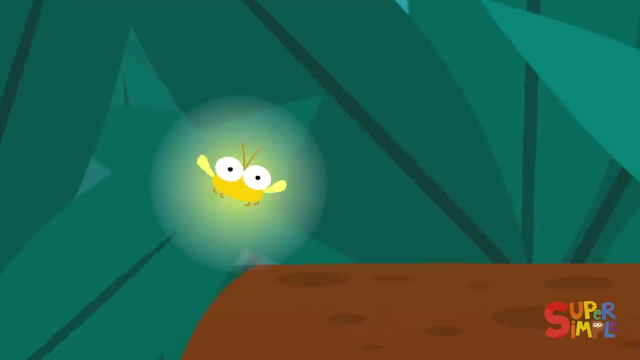 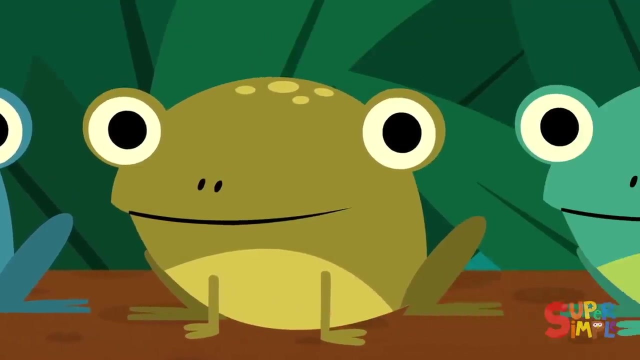 One jumped into the pool, where it was nice and cool. Now there are three green speckled frogs, Glub glub. Three little speckled frogs sat on a speckled log eating some most delicious bugs. Yum, yum. 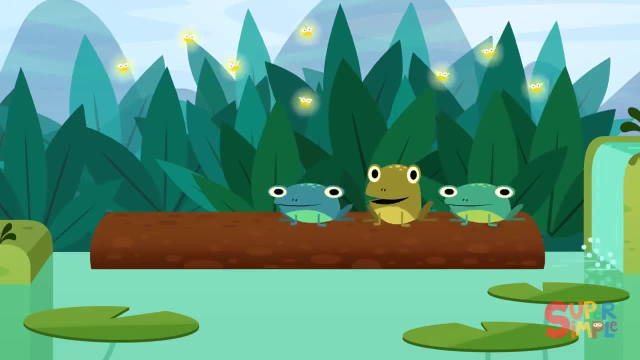 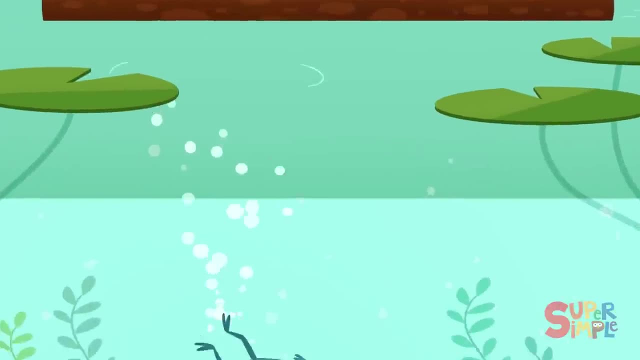 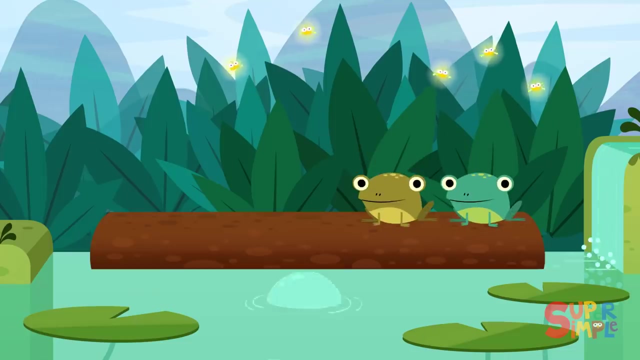 One jumped into the pool, where it was nice and cool. Now there are two green speckled frogs, Glub glub. Four little speckled frogs sat on a speckled log eating some most delicious bugs. Glub glub. 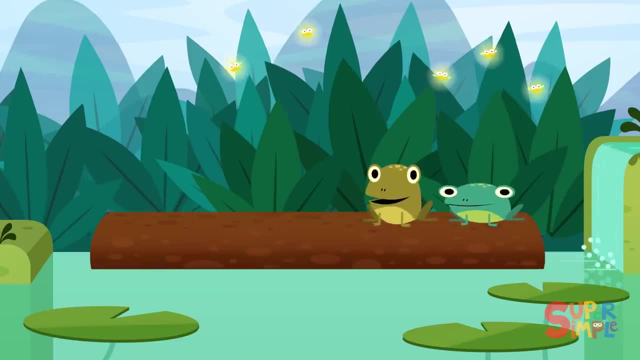 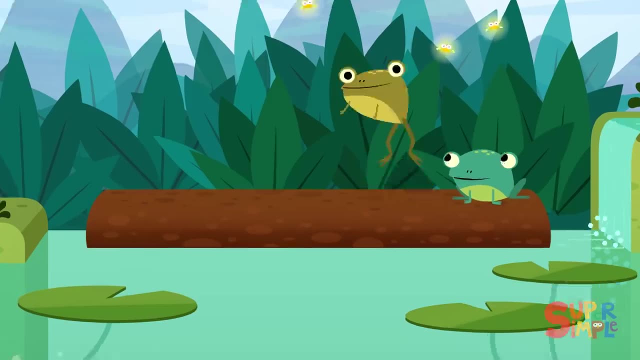 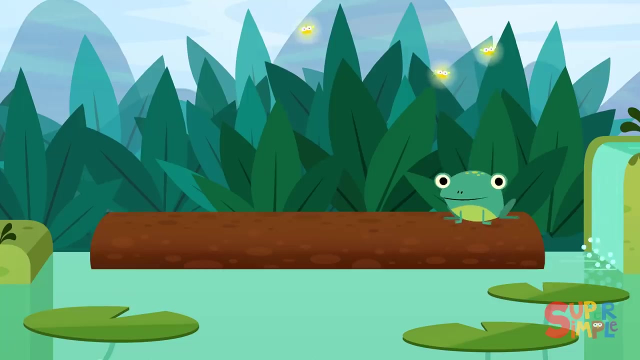 Two little speckled frogs sat on a speckled log eating some most delicious bugs, Yum yum. One jumped into the pool, where it was nice and cool. Now there is one green speckled frog, Glub glub. 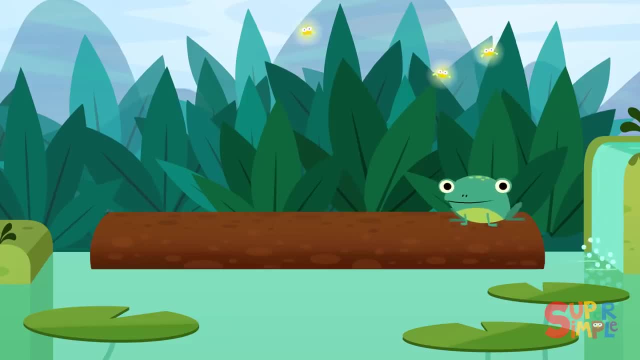 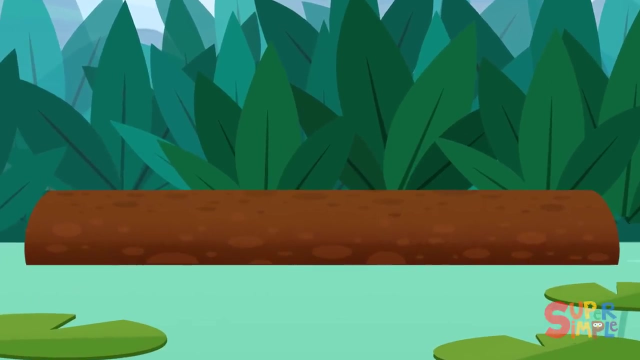 One little speckled frog sat on a speckled log eating some most delicious bugs, Yum yum. One jumped into the pool, where it was nice and cool. Now there are no green speckled frogs. Glub, glub. 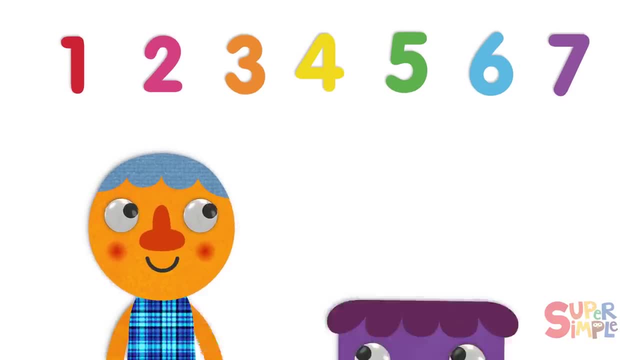 1,, 2,, 3,, 4,, 5,, 6, 7. 1,, 2,, 3,, 4,, 5,, 6, 7. 1,, 2,, 3,, 4,, 5,, 6, 7. 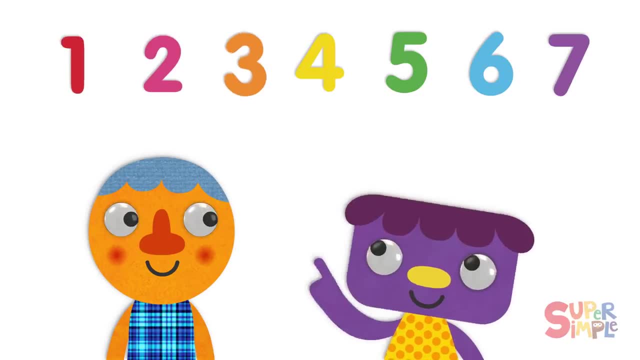 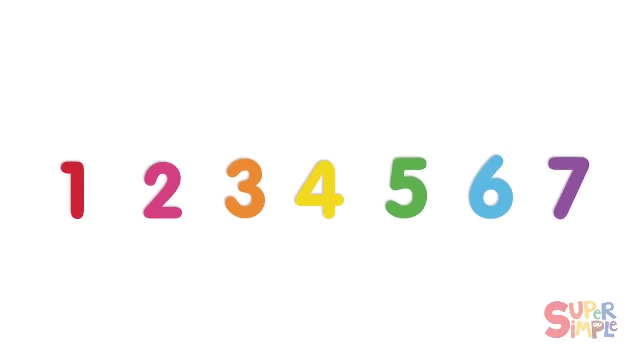 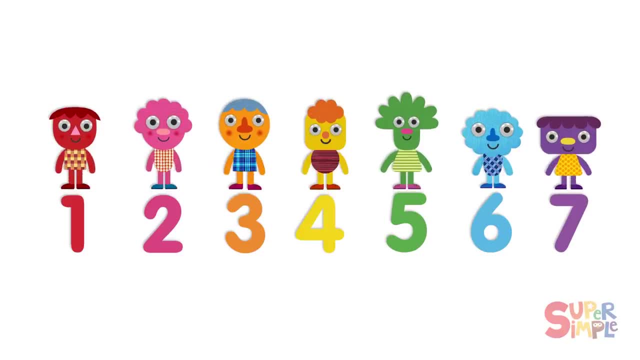 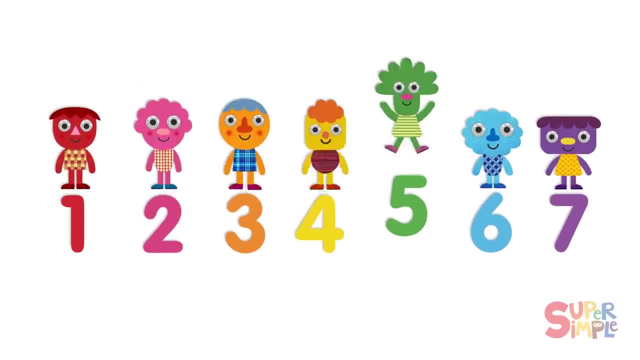 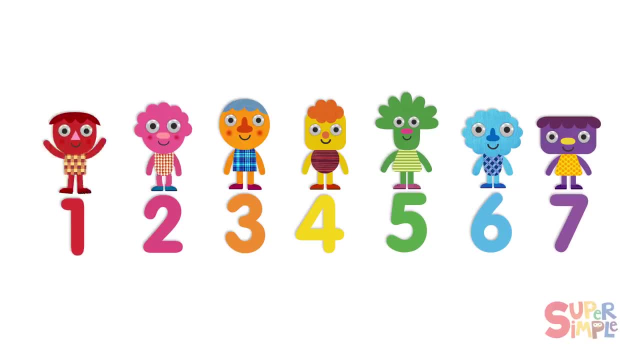 1, 2, 3, 1, 2, 3, 1, 2,, 3,, 4,, 5,, 6, 7. 1, 2,, 3, 1,, 2, 3, 1, 2,, 3,, 4,, 5,, 6, 7. 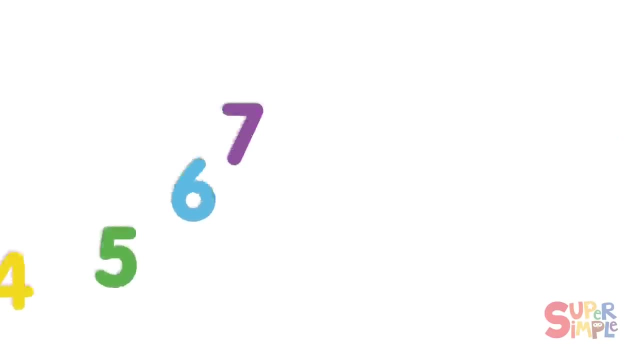 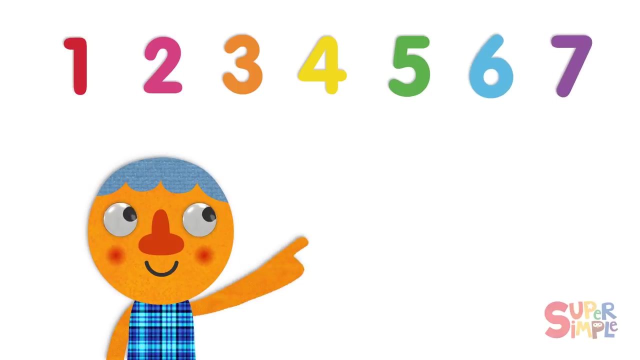 Now let's go backwards, okay: 7, 6,, 5,, 4,, 3,, 2, 1, 7, 6, 5, 4,, 3, 2, 1, 7, 6, 5. 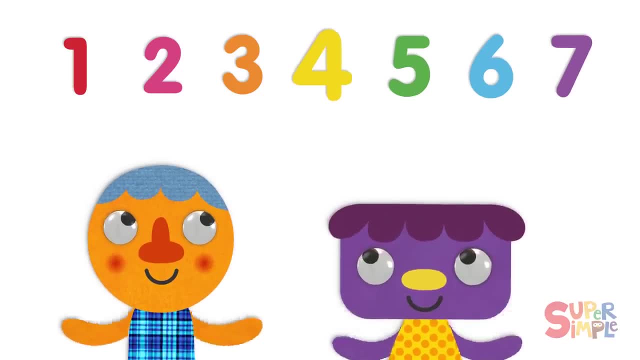 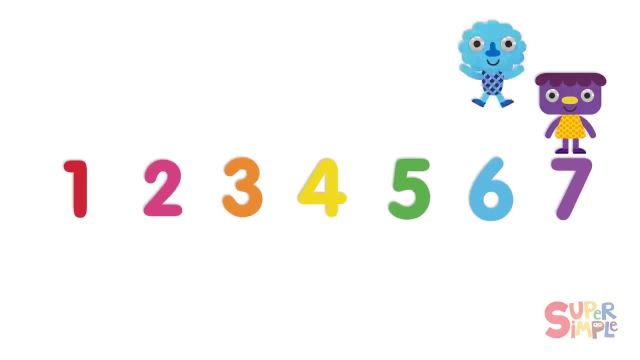 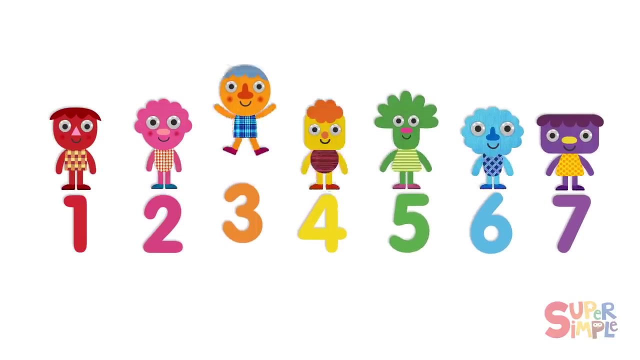 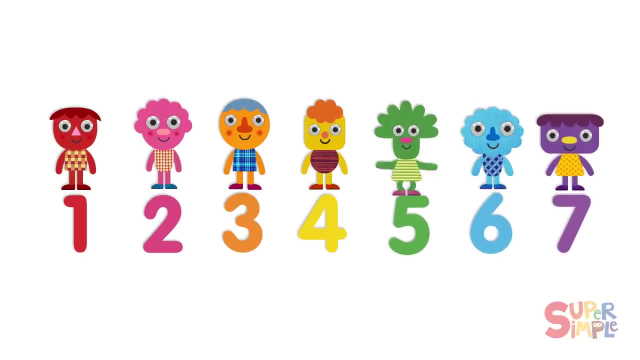 7, 6, 5,, 4,, 3,, 2, 1, 7, 6, 5,, 4, 3, 2, 1, 5, 7, 6, 5, 7, 6, 5,, 4,, 3,, 2, 1. 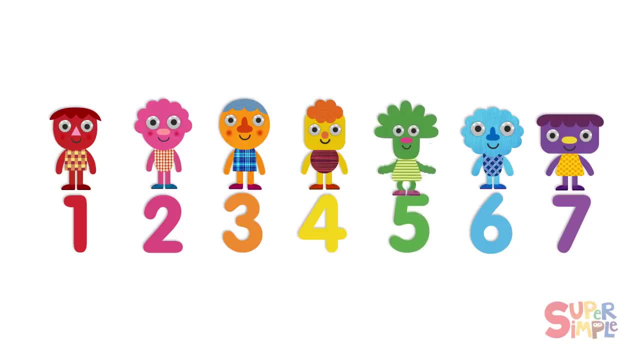 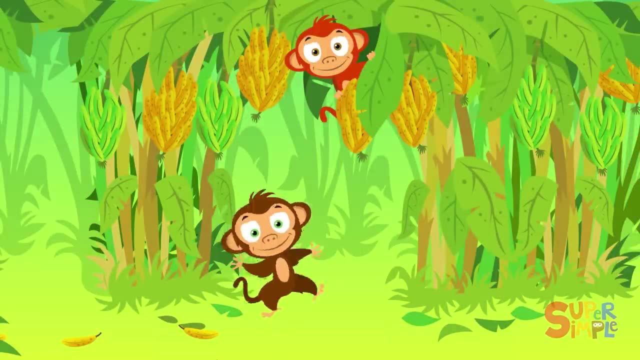 7, 6, 5, 7, 6, 5, 7, 6, 5, 4, 3, 2, 1, 1 banana, 2 bananas 1, 2, 3. 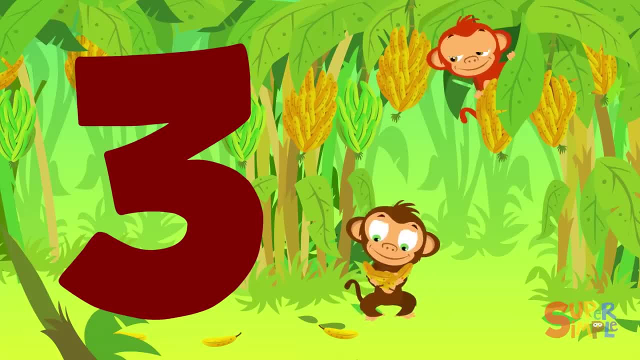 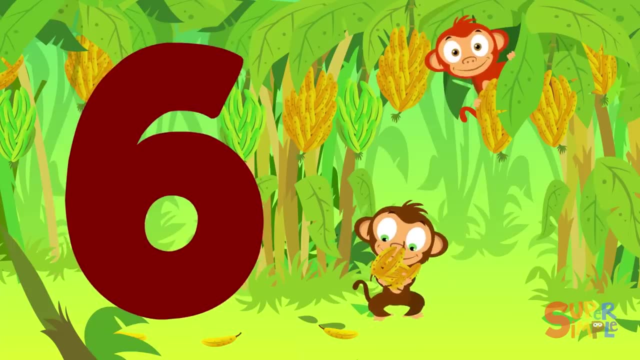 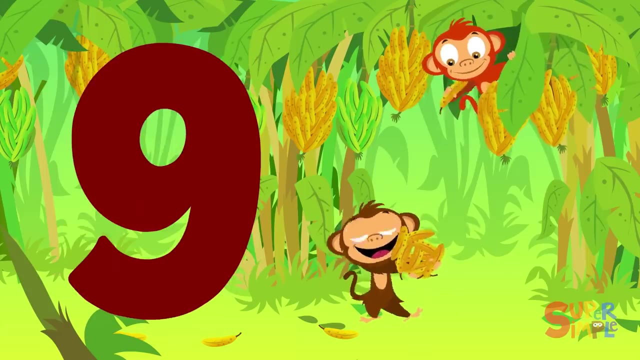 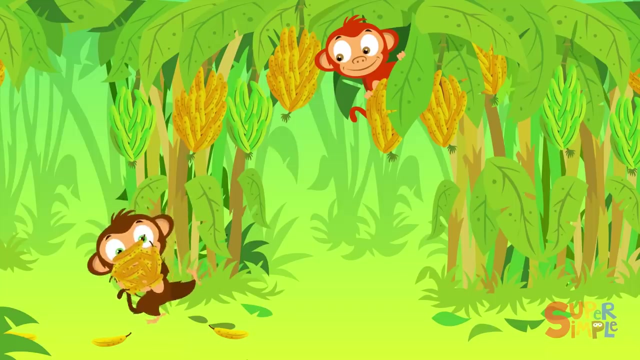 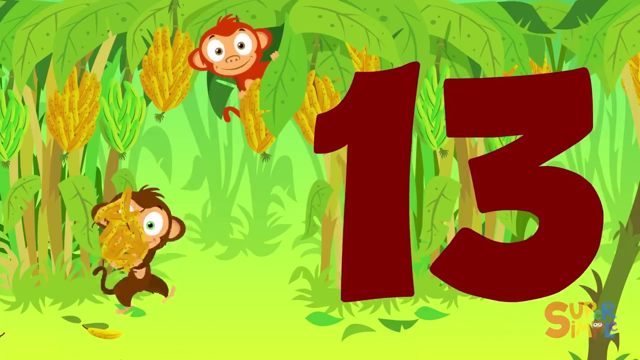 3 bananas for me, 4 bananas, 5 bananas, 4,, 5,, 6, 6 bananas for me, 7,, 8,, 9,, 10, 10 bananas for me, 11,, 12,, 13, 13 bananas for me. 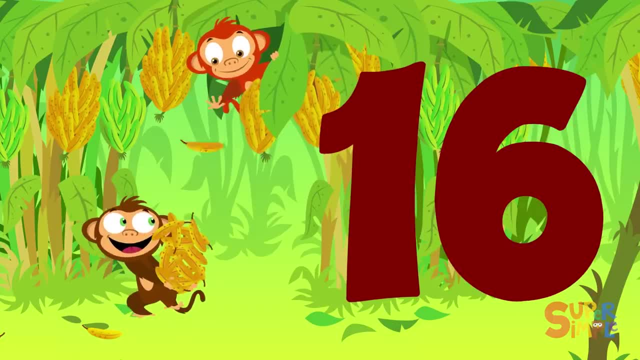 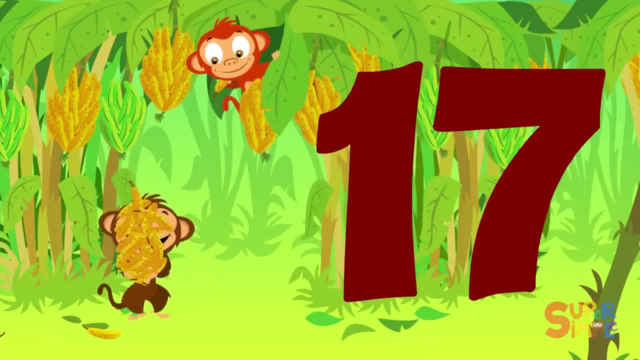 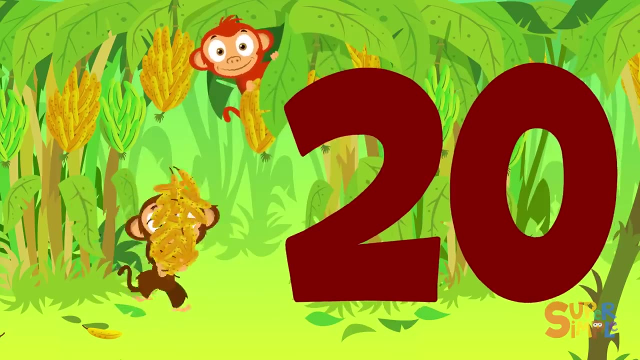 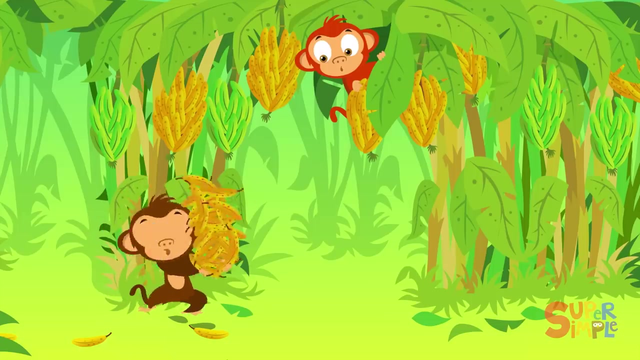 14,, 15,, 16, 16 bananas for me, 17,, 18,, 19, 20,, 20 bananas for me. Bananas to the left. Bananas to the right. Bananas turn around. Bananas turn around. Bananas sit down. 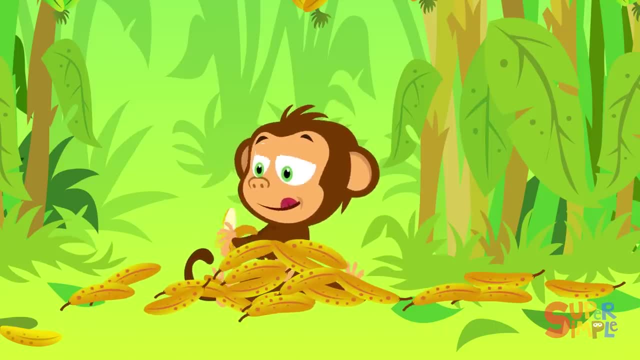 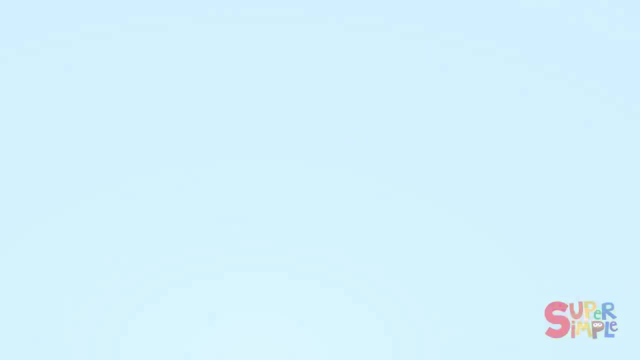 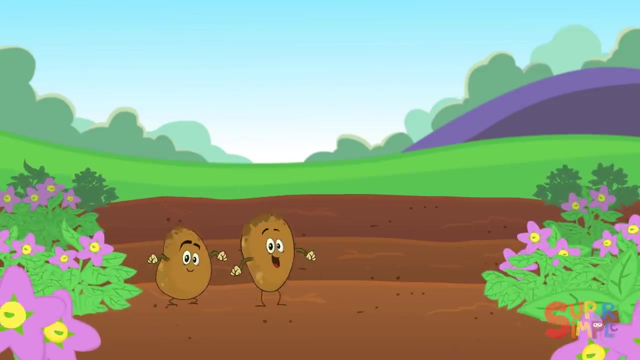 Now peel your bananas and take a bite. One potato, two potatoes, three potatoes, four. One potato, two potatoes, three potatoes, four, Five potatoes, six potatoes, seven potatoes more. One potato, two potatoes, three potatoes, four, Five potatoes, six potatoes, seven potatoes more. 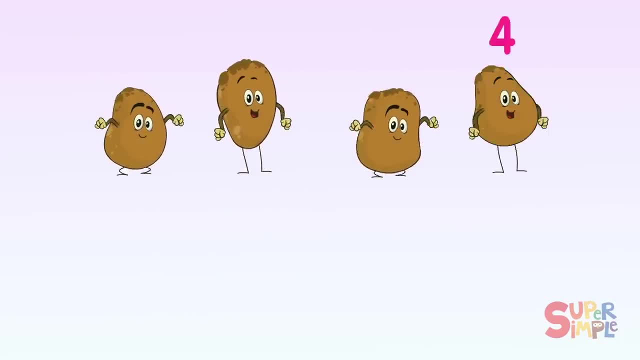 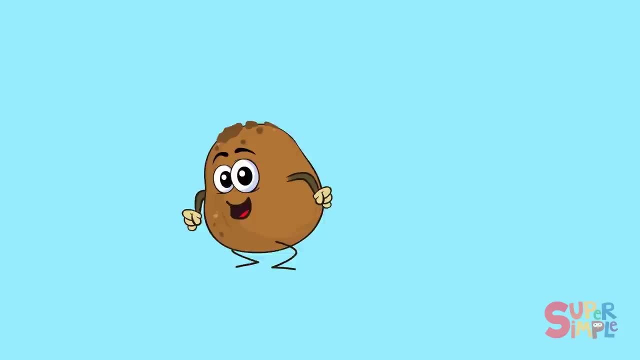 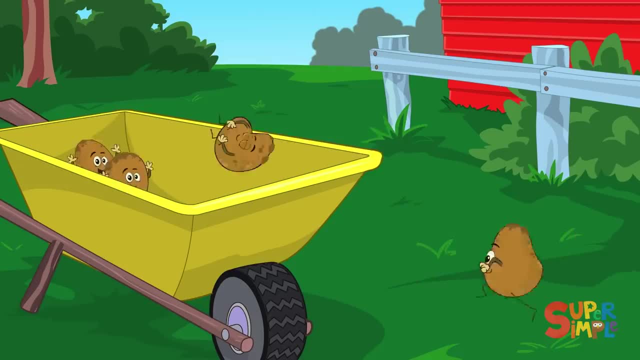 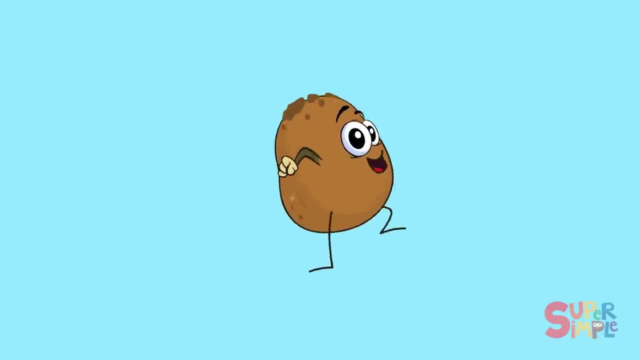 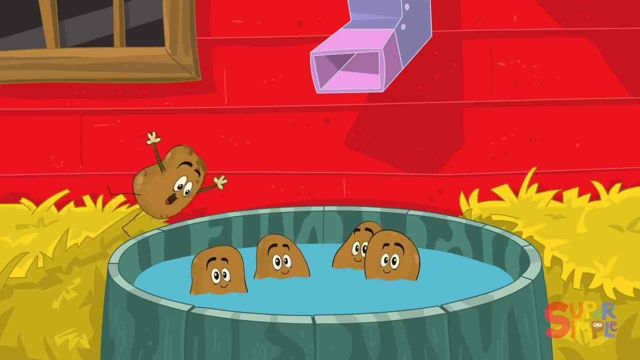 One potato, two potatoes, three potatoes, four, Five potatoes, six potatoes, seven potatoes more. Two potatoes, three potatoes, four, Five potatoes, six potatoes, seven potatoes more. One potato, two potatoes, three potatoes, four, Five potatoes, six potatoes, seven potatoes more. 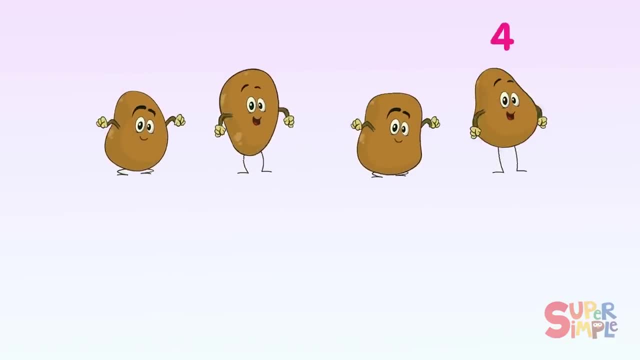 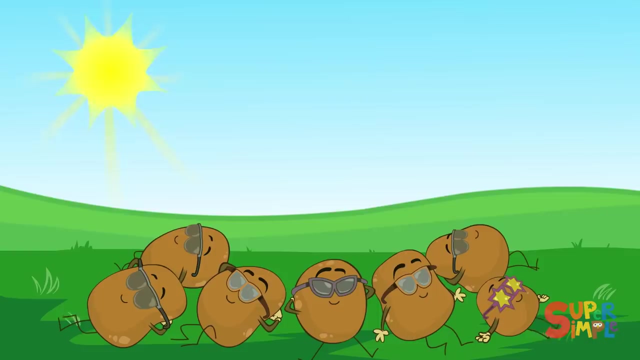 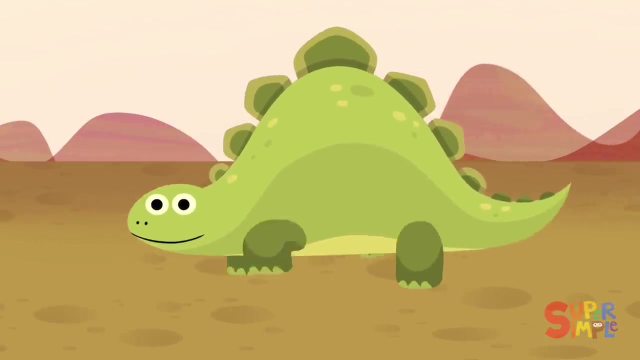 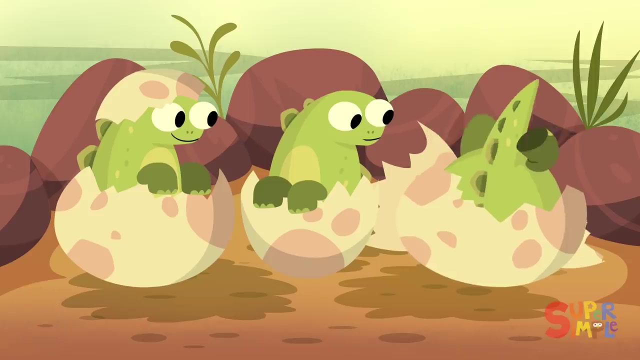 One potato, two potatoes, three potatoes, four, Five potatoes, six potatoes, seven potatoes more. One potato, two potatoes, three potatoes, four, Five potatoes, six potatoes, seven potatoes more. Stegosaurus: One little, two little, three little dinosaurs. 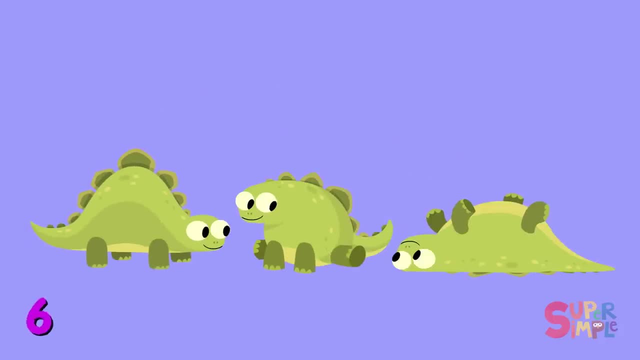 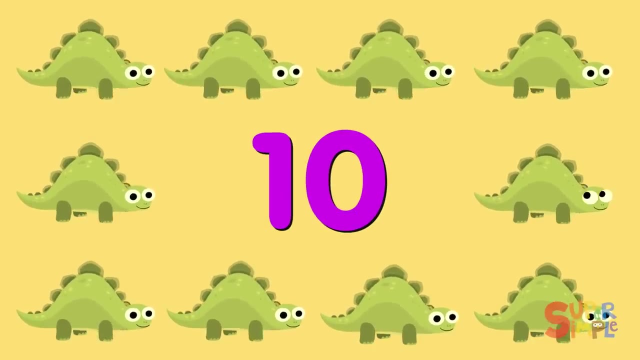 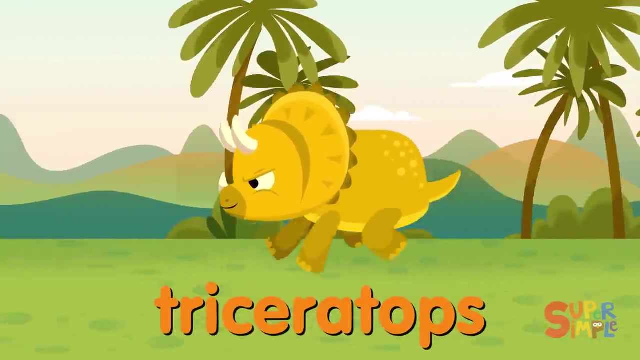 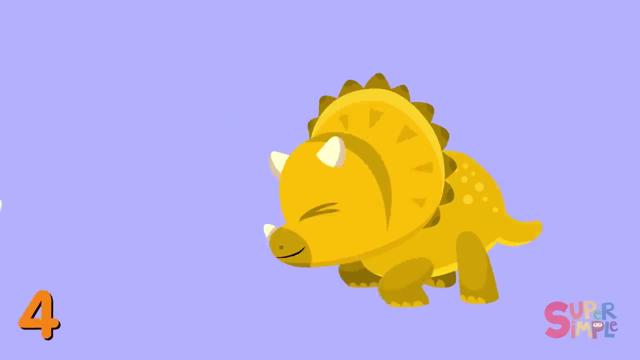 Four little, five little, six little dinosaurs. Seven little, eight little, nine little dinosaurs. Ten little dinosaur babies. Triceratops. One little, two little, three little dinosaurs. Four little, five little, six little dinosaurs. Seven little, eight little, nine little dinosaurs. 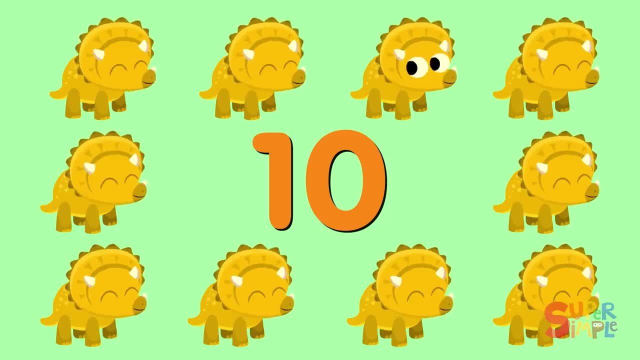 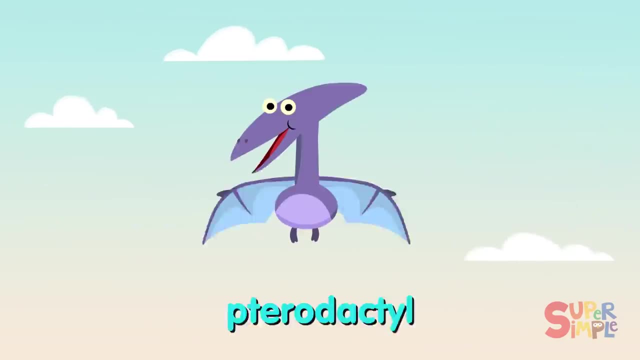 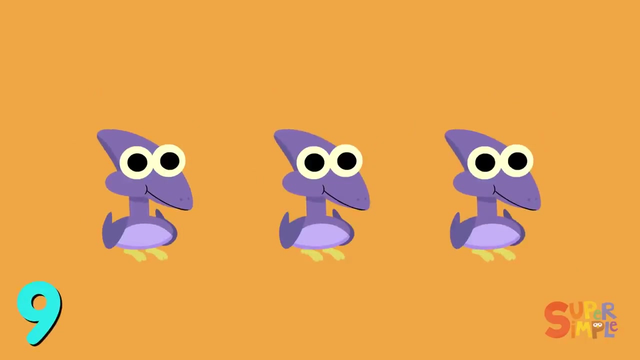 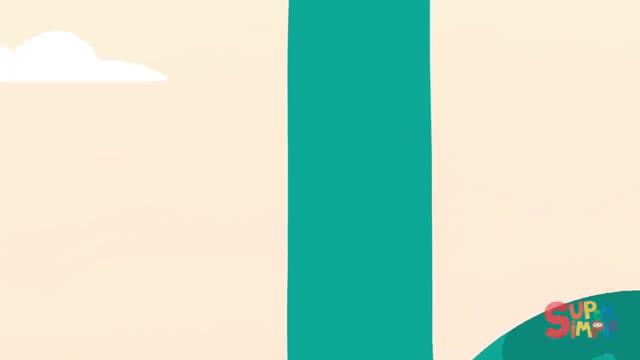 Nine little dinosaurs, Ten little dinosaur babies. Pterodactyl. One little, two little, three little dinosaurs Four little, five little, six little dinosaurs. Seven little, eight little, nine little dinosaurs. Ten little dinosaur babies, Tyrannosaurus. Tyrannosaurus. 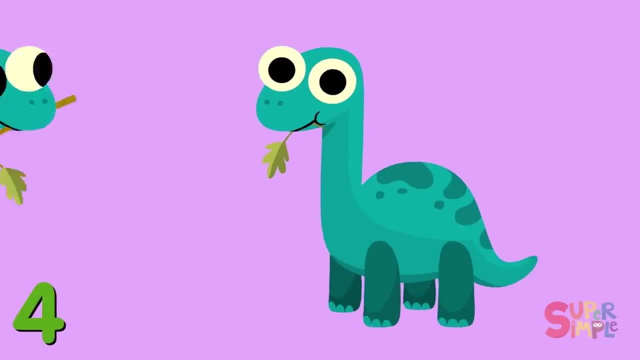 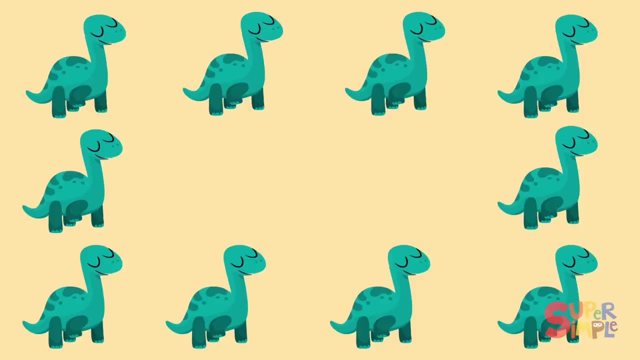 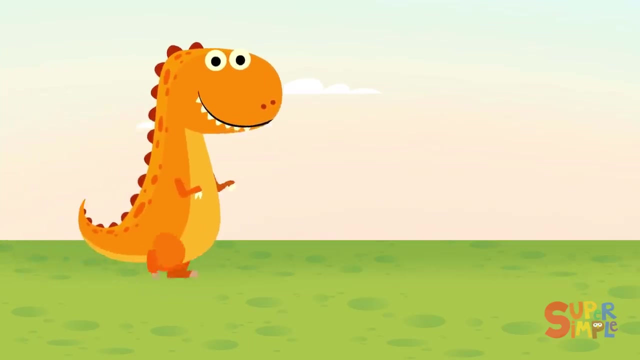 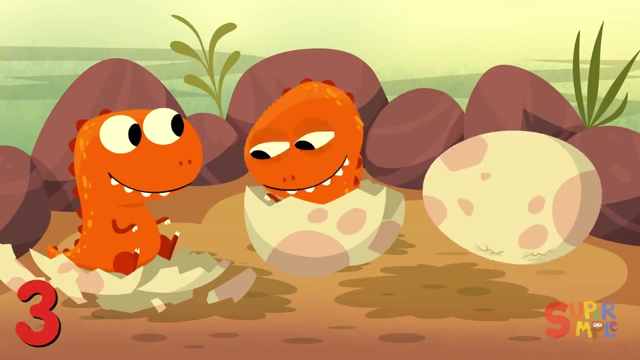 One little, two little, three little dinosaurs. Four little, five little, six little dinosaurs. Seven little, eight little, nine little dinosaurs. Ten little dinosaur babies. Tyrannosaurus Rex. One little, two little, three little dinosaurs. Four little, five little, six little dinosaurs. 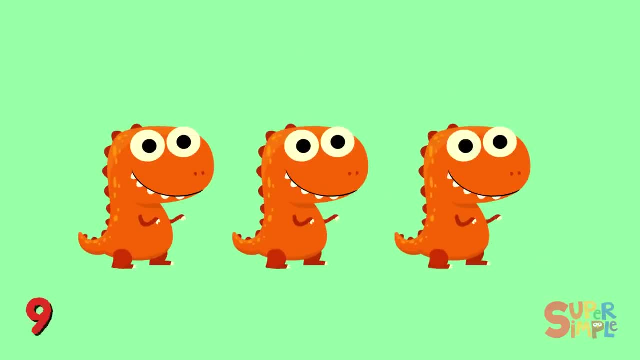 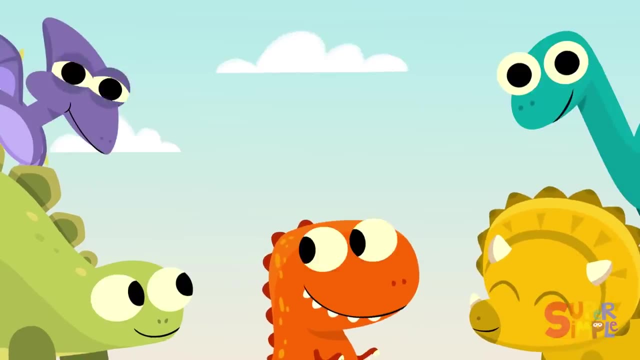 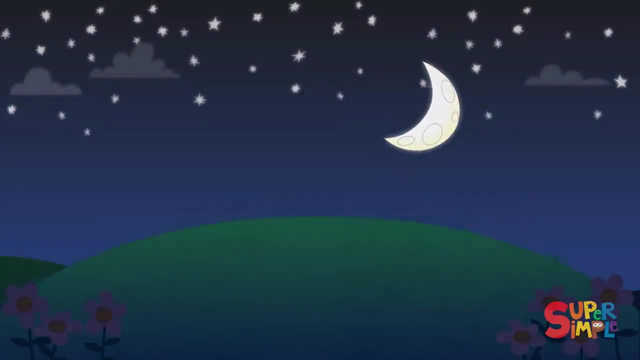 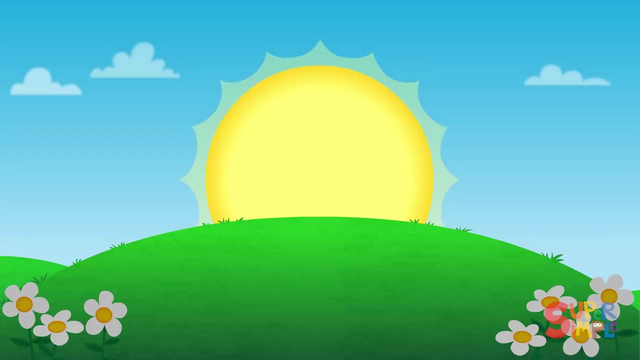 Seven little eight. little nine little dinosaurs, Ten little dinosaur babies. Let's get started with some counting. Can you count to twenty? Here we go. One, two, three, four, five, six, Seven, eight, nine, ten, Eleven, twelve, thirteen. 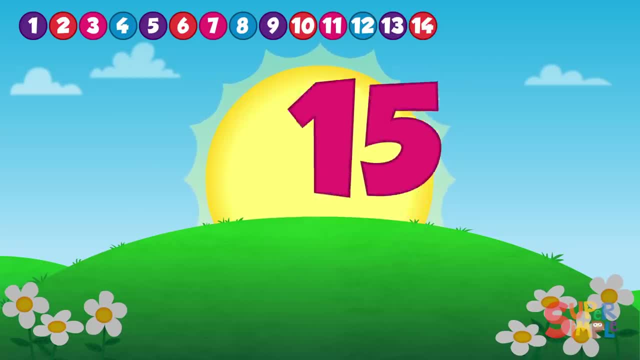 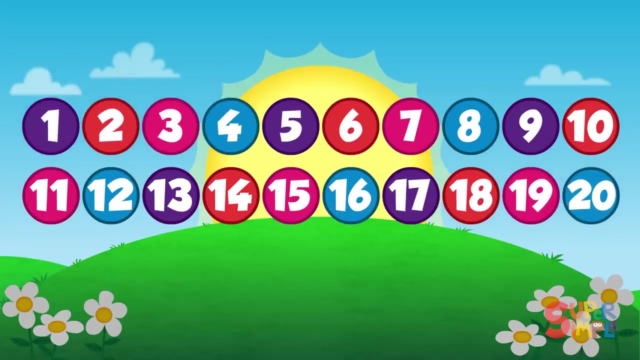 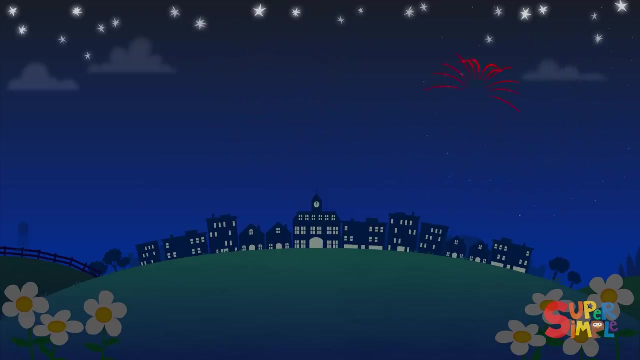 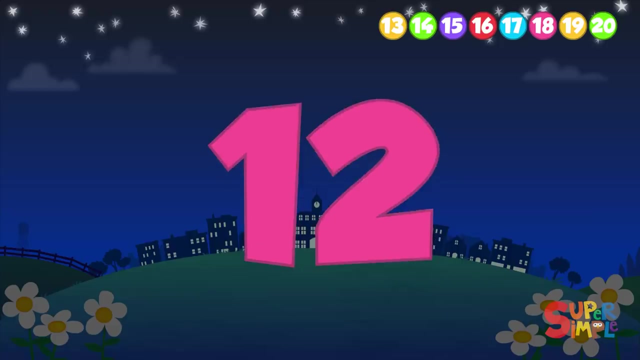 Fourteen, fifteen, sixteen, Seventeen, eighteen, nineteen, twenty. That was fun. Let's count down from twenty. Are you ready? Here we go. Twenty, Nineteen, eighteen, seventeen, Sixteen, fifteen, fourteen, Thirteen, twelve, eleven. 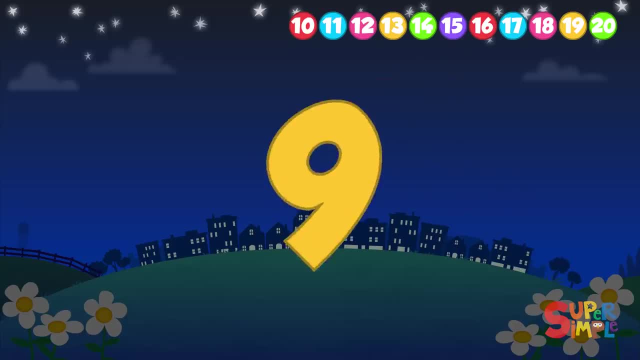 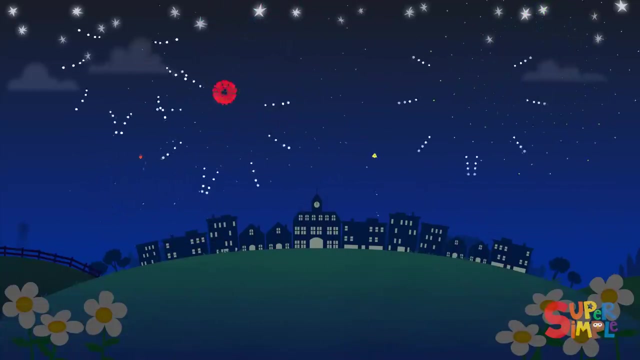 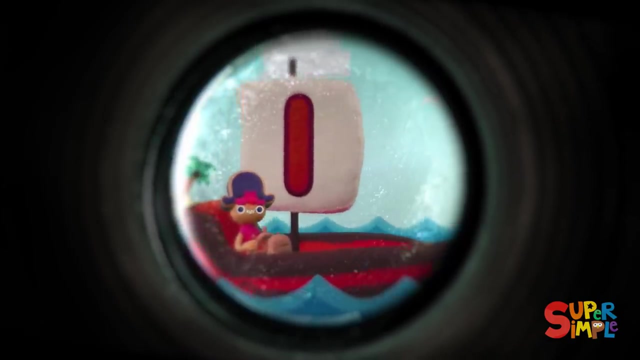 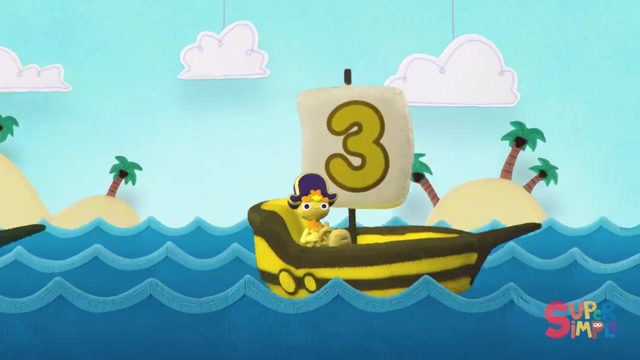 Ten, nine, eight, Seven, six, five, Fourteen, fifteen, sixteen, sixteen, Six, One, Two, Three, Two, One. We did it, Crazy KAZAtier. One little, two little, three little sailboats, Four little, five little, six little sailboats. 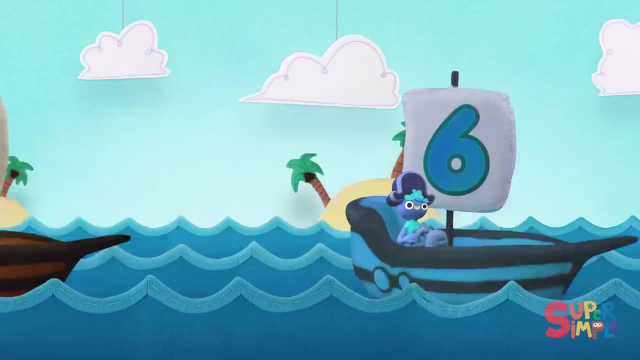 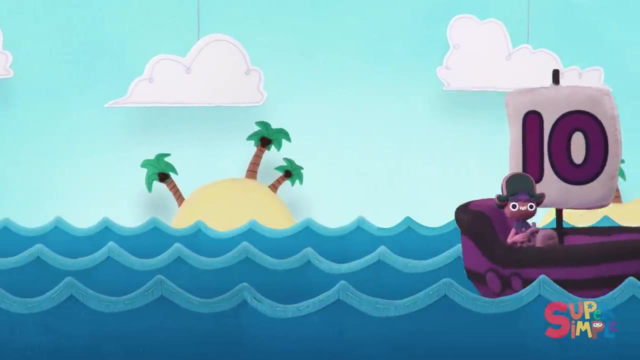 Nine little, ten little, eleven little sailboats, Sixteen little, twelve little, sixteen little sailsboats, Seven little, ten little, eleven little sailboats. Sailboats seven little, eight little, nine little sailboats, ten little sailboats. Great job, guys. now Let's count them backwards. 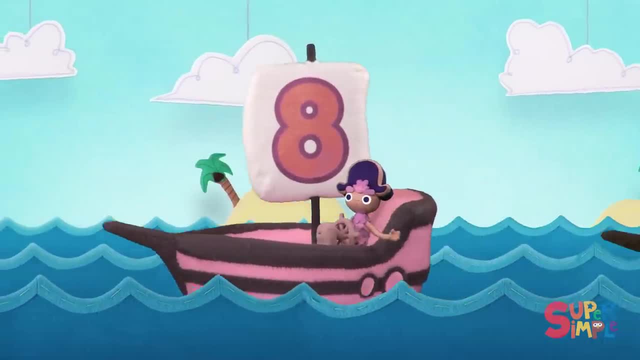 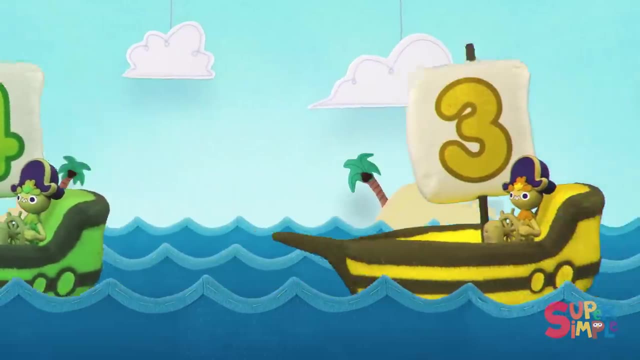 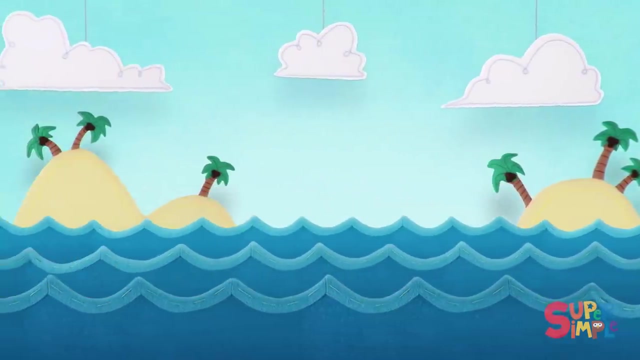 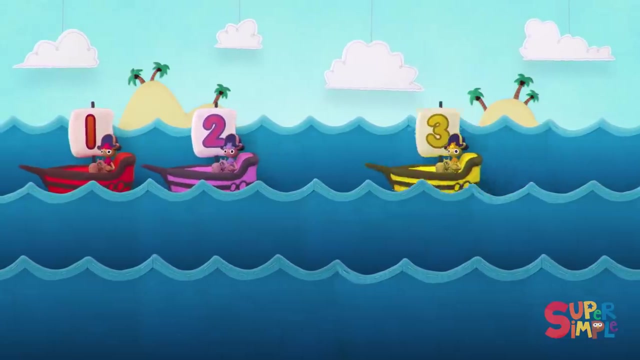 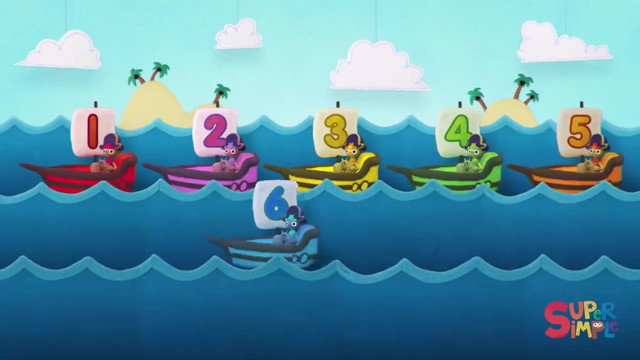 Ten little, nine little, eight little sailboats, seven little, six little, five little sailboats, four little, three little two little sailboats, one little sailboat, One sailboat, two sailboats, three sailboats, four sailboats, five sailboats, six sailboats, seven sailboats, eight sailboats. 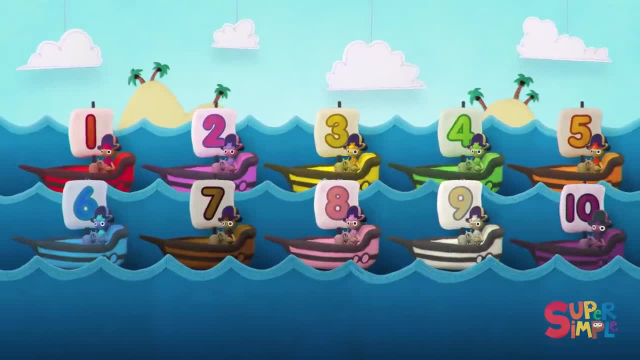 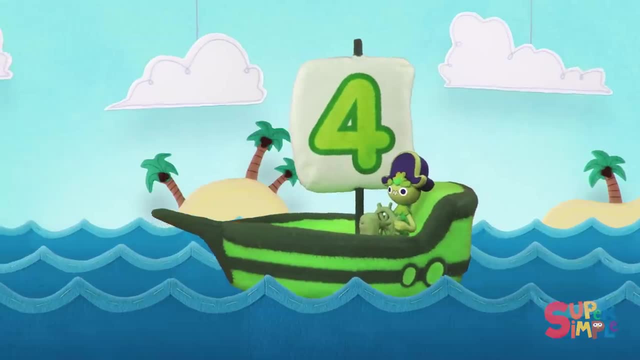 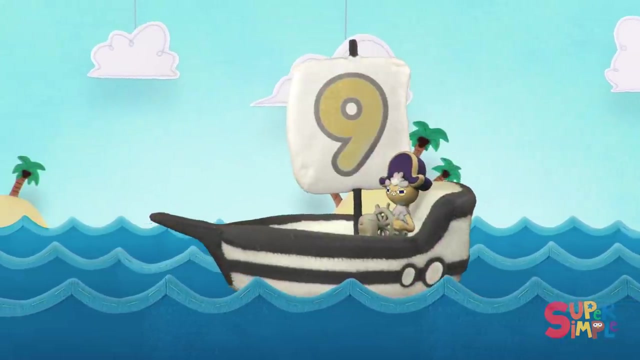 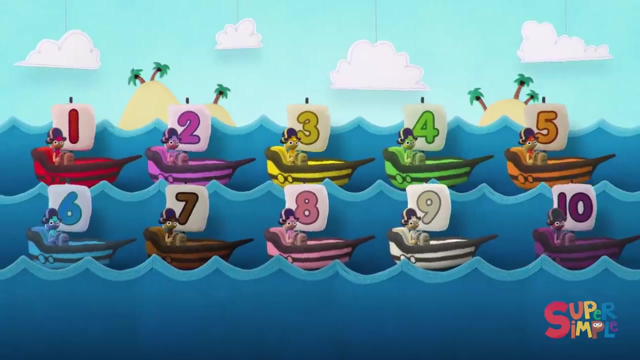 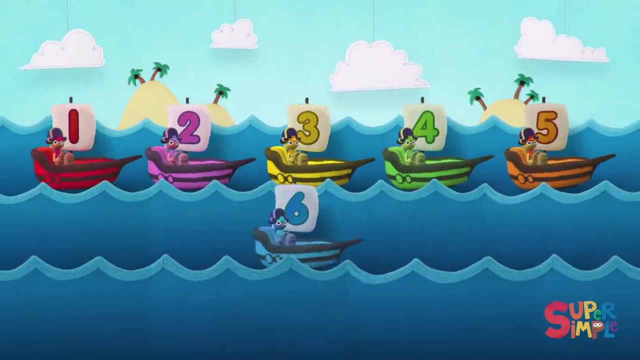 nine sailboats, ten sailboats: One little, two, little three, let's two sail from four Little, five little little sailboat seven, little, eight, little nine. little sailboat, 10 little sailboats backwards: Ten little nine, eight little sailboat little, six, little five little sails go. 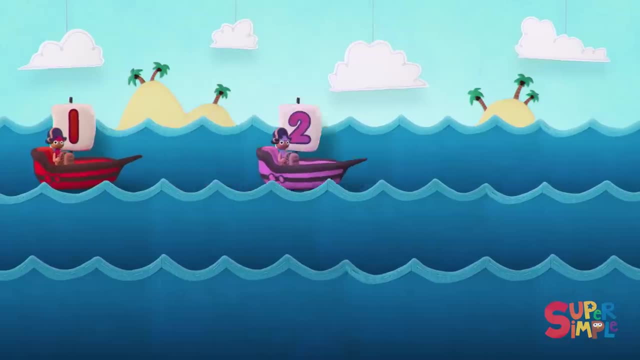 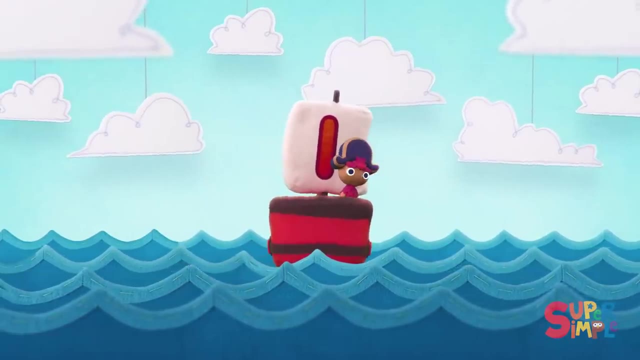 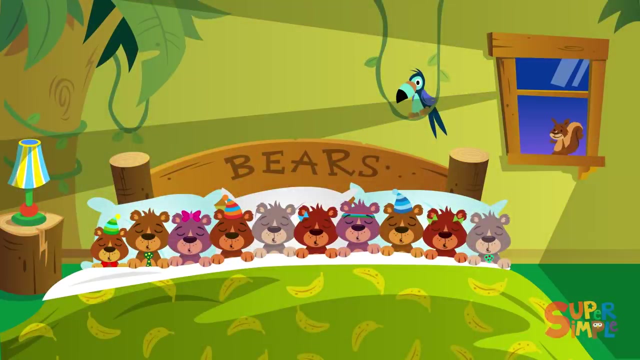 Four little, three little, two little sailboats. One little sailboat. That was fun. Thanks for counting with me. Here we go. There were ten in the bed And the little one said: Roll over, roll over. So they all rolled over And one fell out. 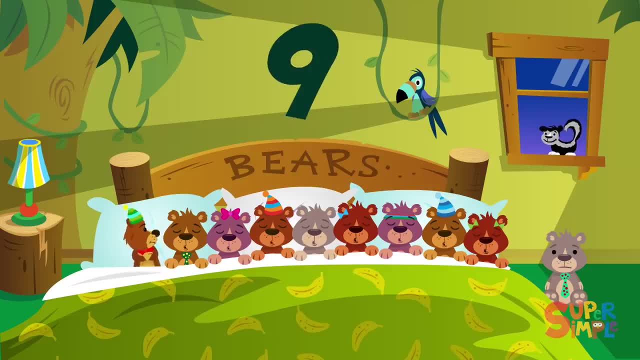 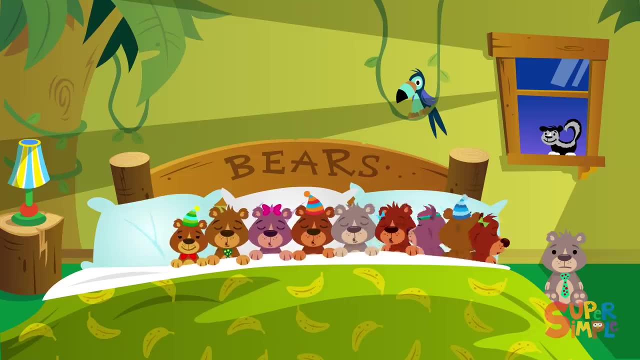 There were nine in the bed And the little one said, Roll over, roll over. So they all rolled over And one fell out. There were eight in the bed And the little one said, Roll over, roll over. So they all rolled over And one fell out. 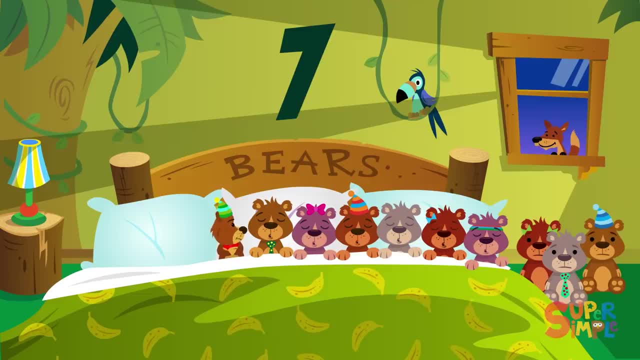 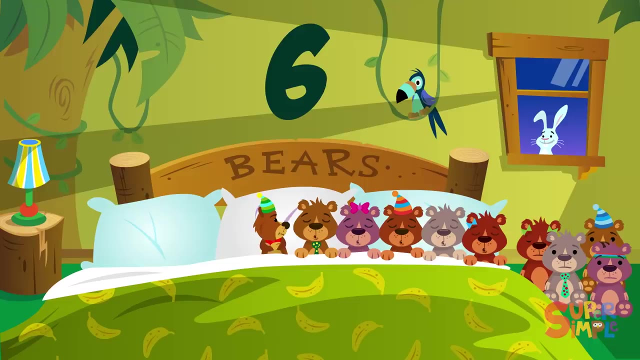 There were seven in the bed And the little one said, Roll over, roll over. So they all rolled over And one fell out. There were six in the bed And the little one said, Roll over, roll over. So they all rolled over And one fell out. 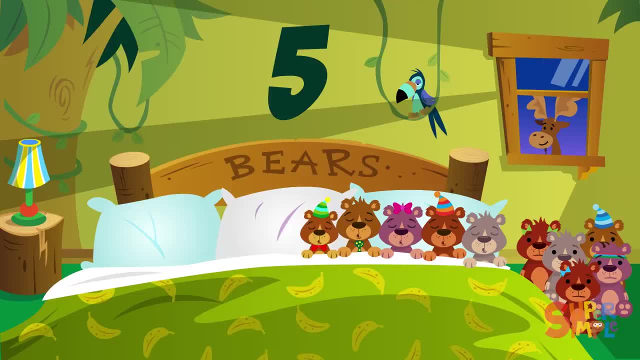 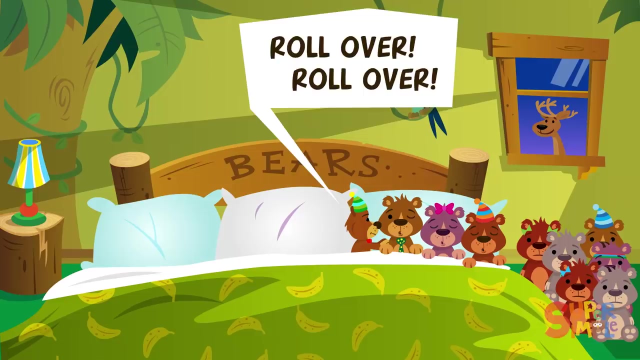 There were five in the bed And the little one said, Roll over, roll over. So they all rolled over And one fell out. There were four in the bed And the little one said, Roll over, roll over. So they all rolled over And one fell out. 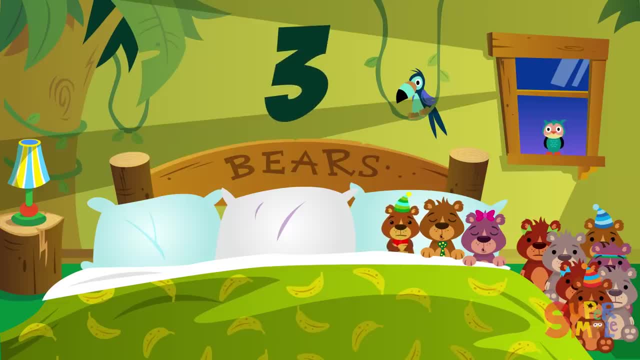 There were three in the bed And the little one said, Roll over, roll over. So they all rolled over And one fell out. There were two in the bed And the little one said, Roll over, roll over. So they both rolled over And one fell out. 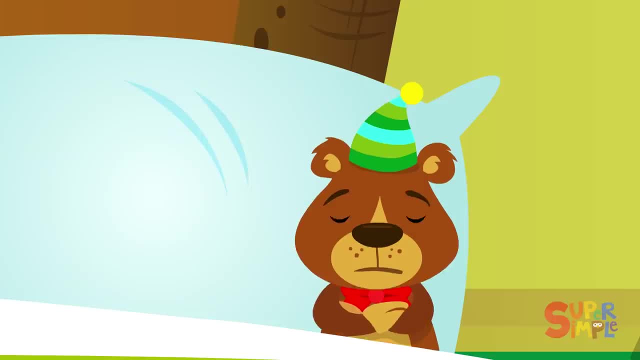 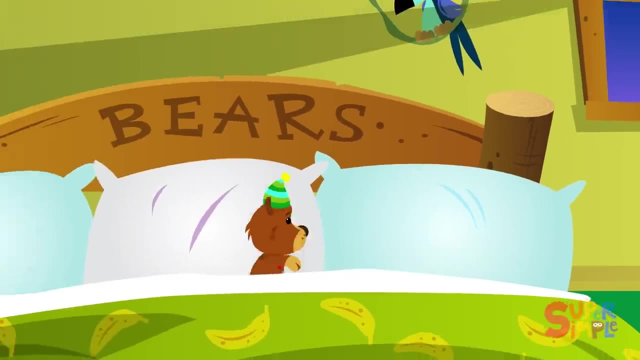 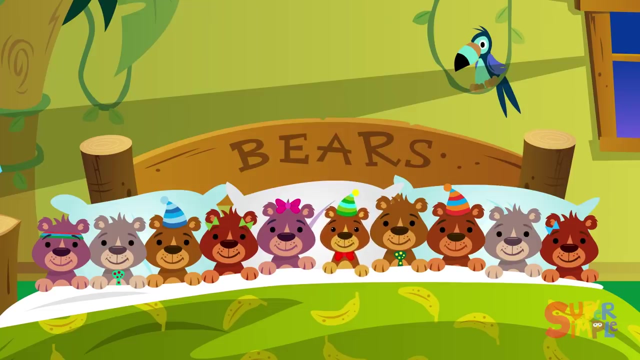 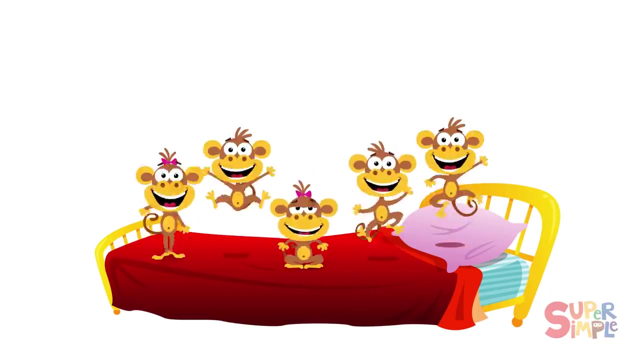 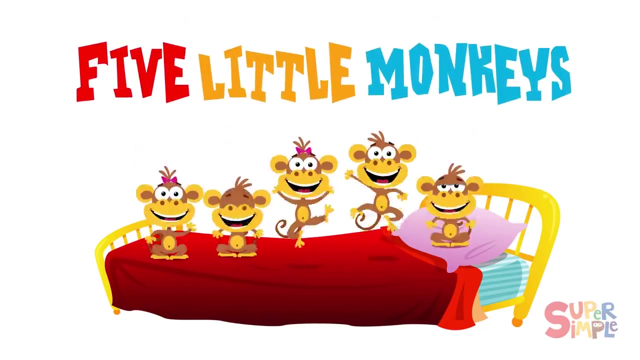 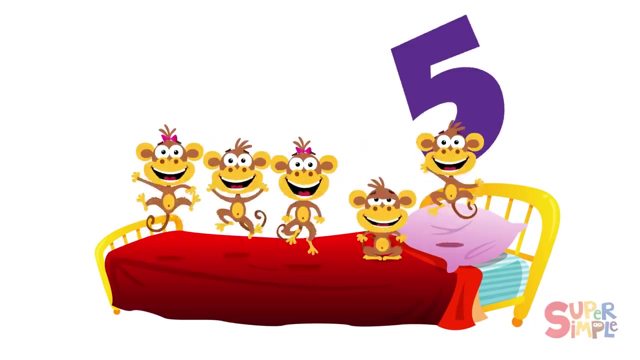 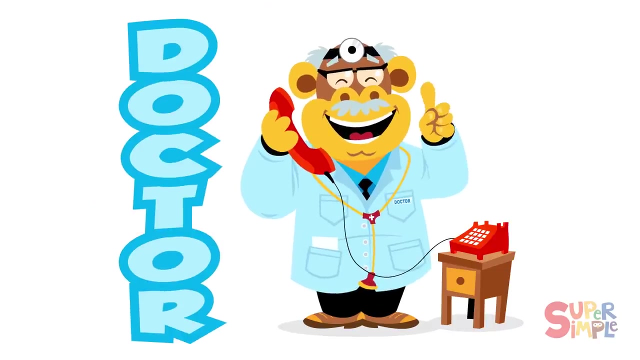 There was one in the bed And the little one said I'm lonely. And the little one said I'm lonely. Five little monkeys jumping on the bed. One fell off and bumped his head. Mama called the doctor and the doctor said: No more monkeys jumping on the bed. 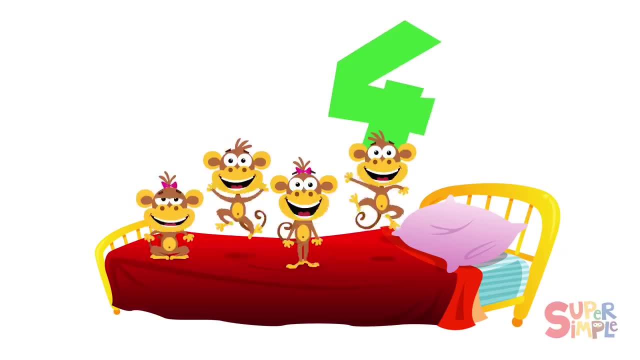 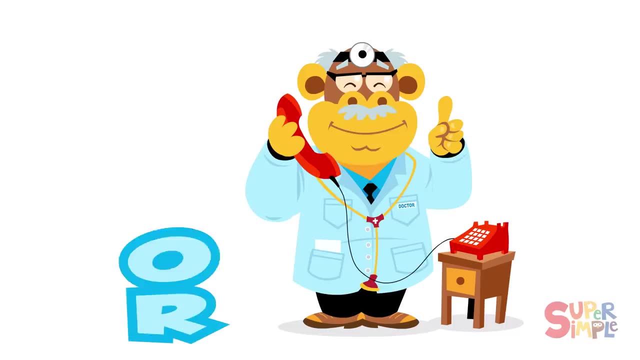 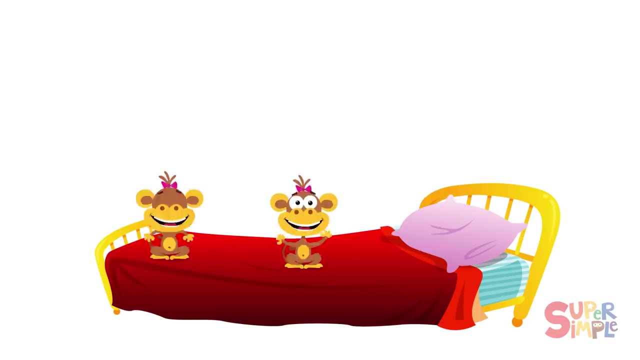 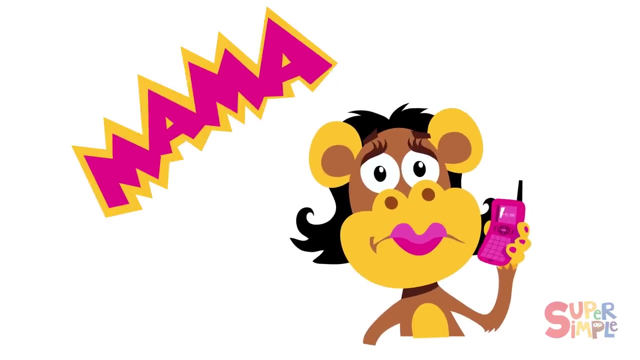 Four little monkeys jumping on the bed. One fell off and bumped his head. Mama called the doctor and the doctor said: No more monkeys jumping on the bed. Three little monkeys jumping on the bed. One fell off and bumped her head. Mama called the doctor and the doctor said: 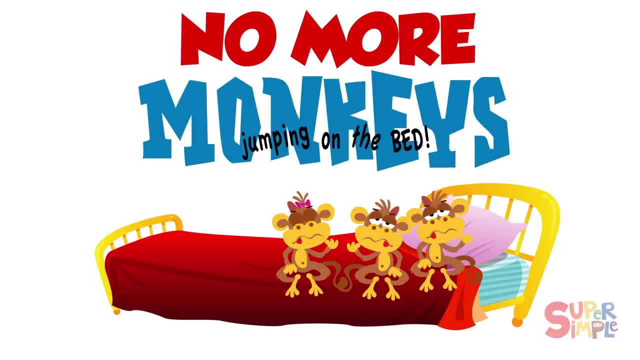 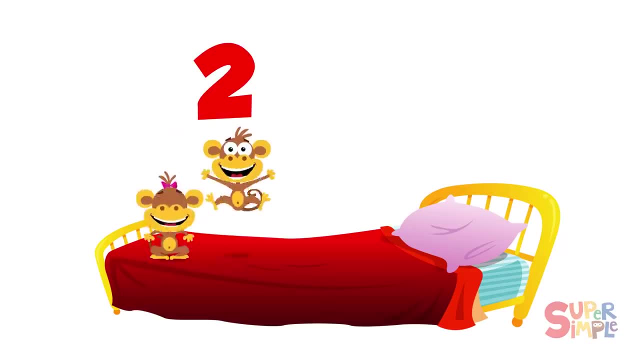 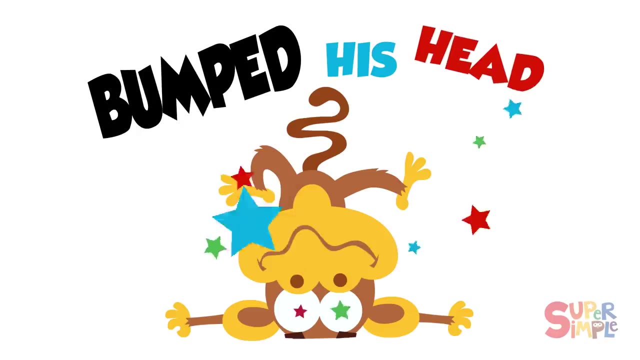 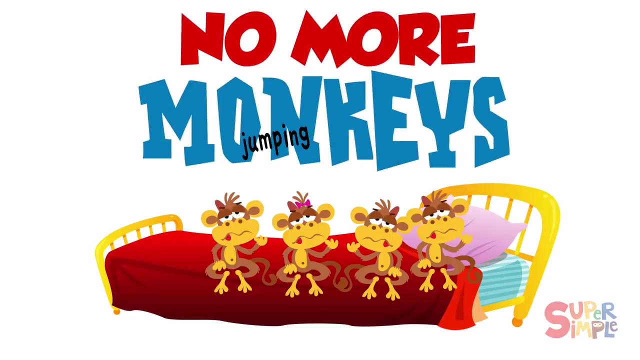 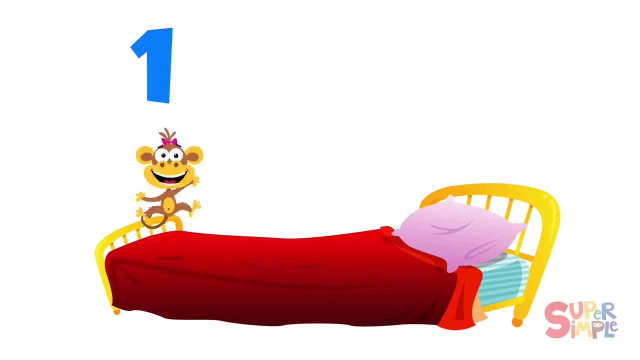 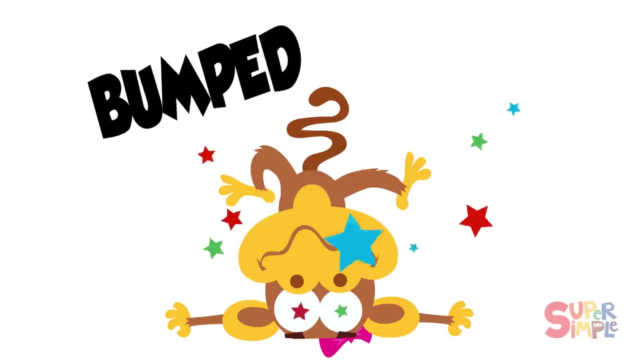 No more monkeys jumping on the bed. Two little monkeys jumping on the bed. One fell off and bumped his head. Mama called the doctor and the doctor said: No more monkeys jumping on the bed. One little monkey jumping on the bed. She fell off and bumped her head. Mama called the doctor and the doctor said: 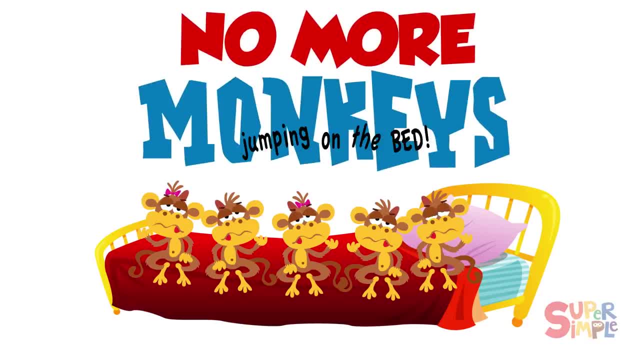 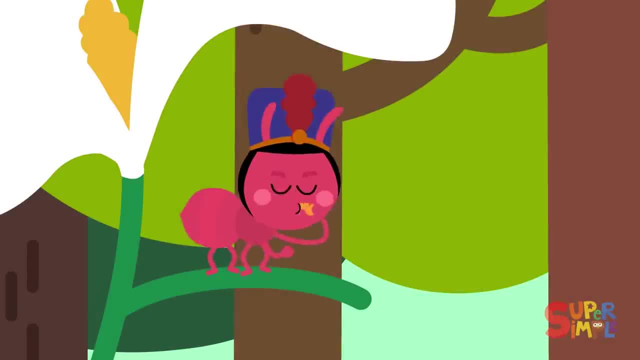 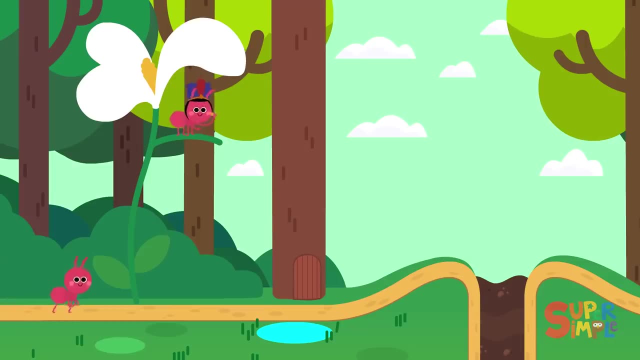 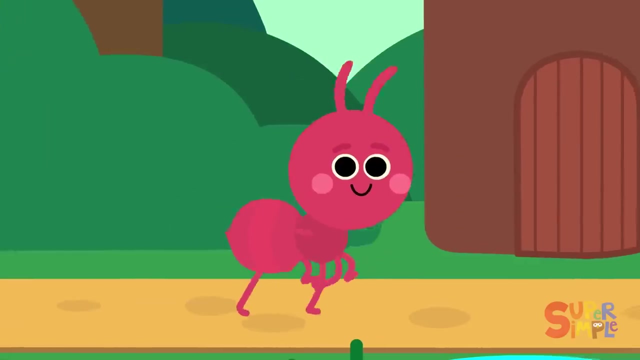 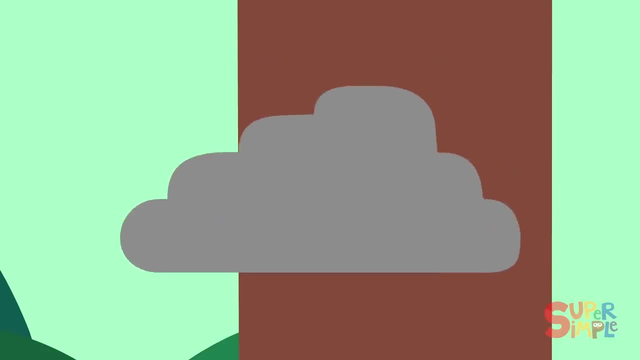 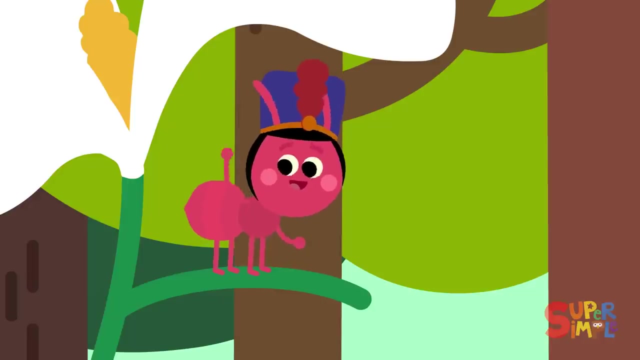 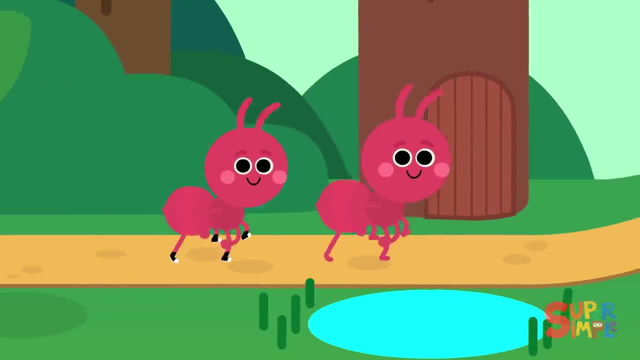 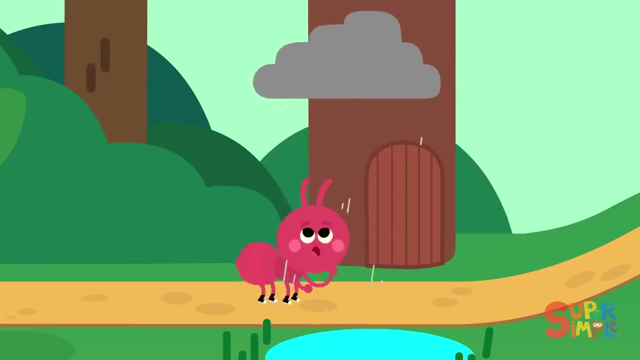 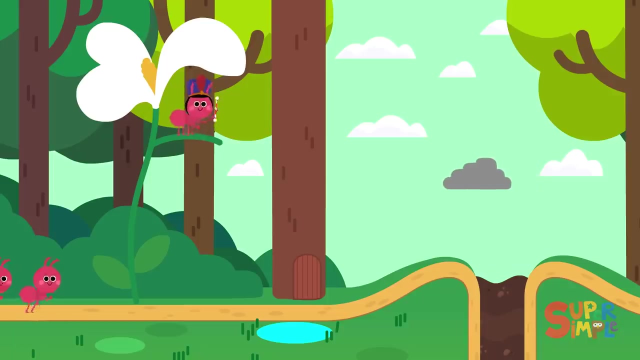 One little monkey jumping on the bed. One little monkey jumping on the bed. The ants go marching 2 by 2. The little one stops to tie his shoe And they all go marching down To the ground to get out of the rain. Boom, Boom, Boom, The ants go marching three by three. 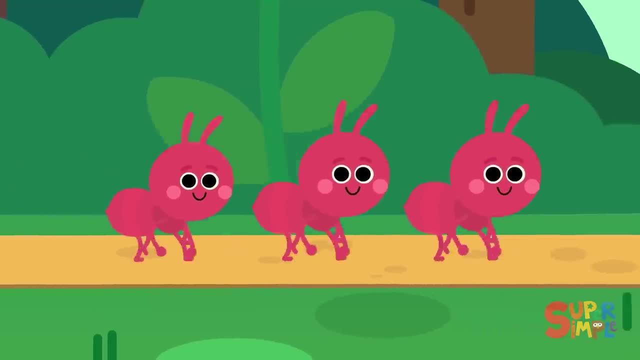 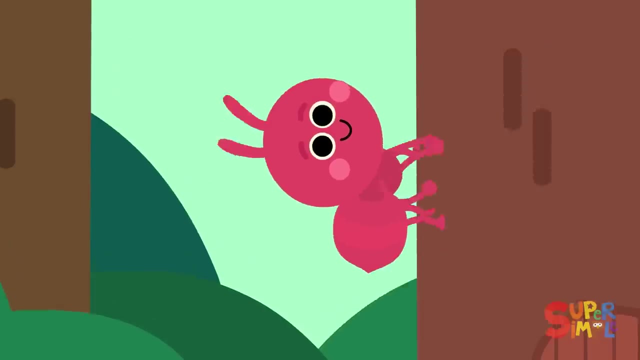 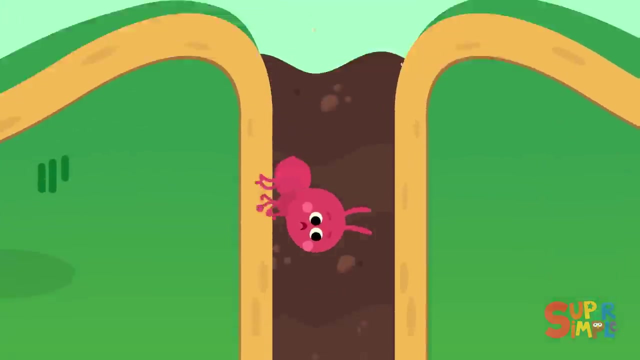 Hurrah, Hurrah, The ants go marching 3 by 3. Hurrah, Hurrah, The ants go marching 3 by 3. The little one stops to climb a tree And they all go marching down To the ground to get out of the rain. Boom, boom, boom. 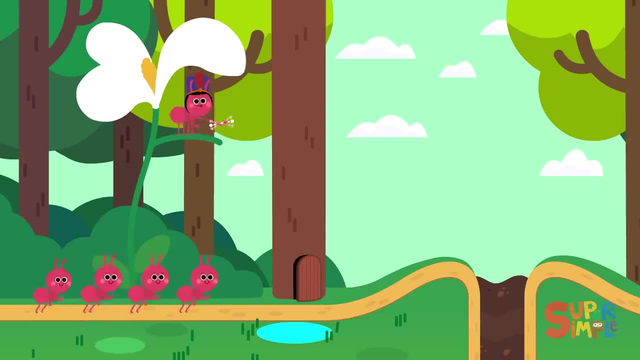 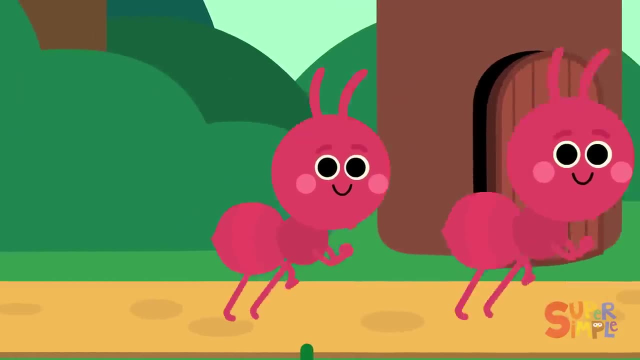 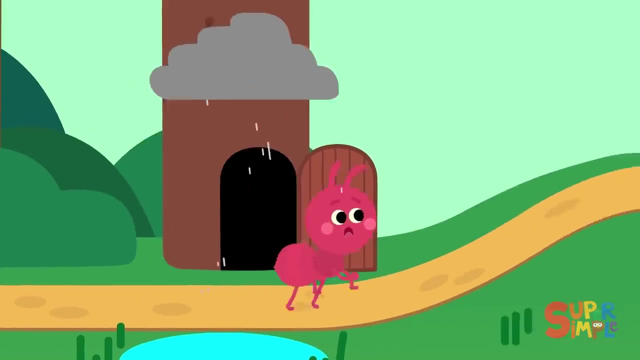 The ants go marching four by four. Hurrah, hurrah. The ants go marching four by four. Hurrah, hurrah. The ants go marching four by four. The little one stops to shut the door And they all go marching down To the ground to get out of the rain. 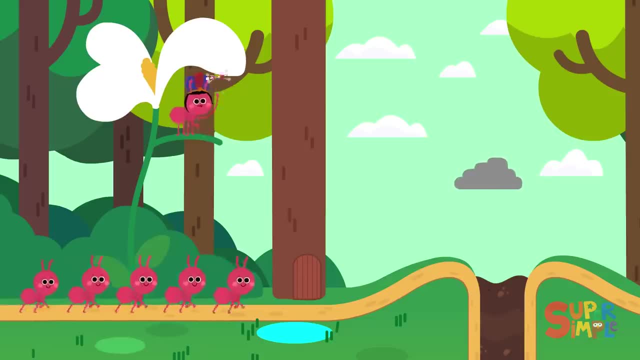 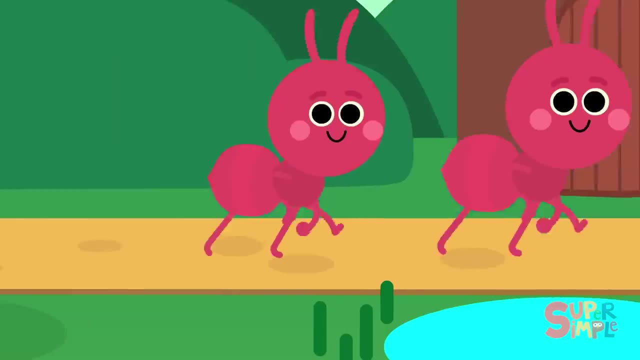 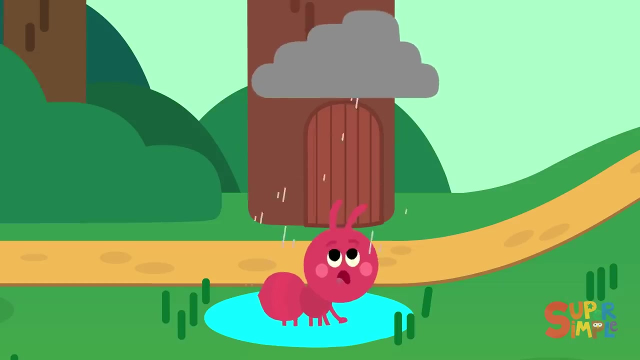 Boom, boom, boom. The ants go marching five by five. Hurrah, hurrah. the ants go marching five by five. Hurrah, hurrah. the ants go marching five by five. The little one stops to take a dive and they all go marching down to the ground to get out of the rain. 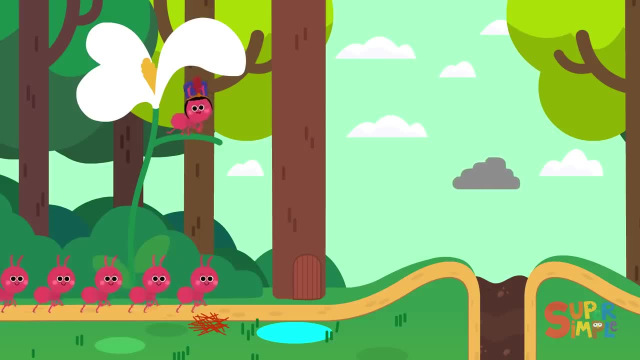 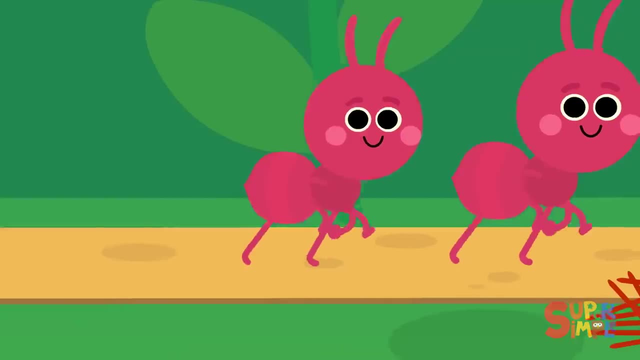 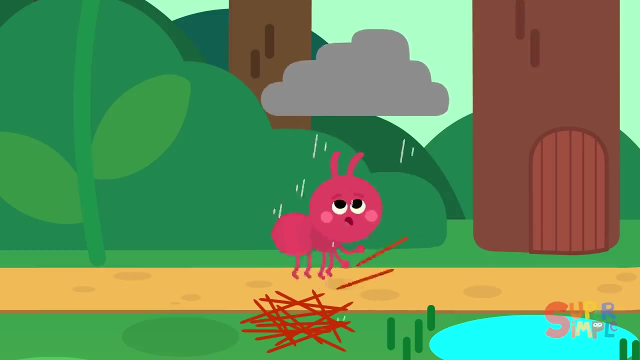 Boom, boom, boom. the ants go marching six by six. Hurrah, hurrah. the ants go marching six by six. Hurrah, hurrah. the ants go marching six by six. The little one stops to pick up sticks and they all go marching down to the ground to get out of the rain. 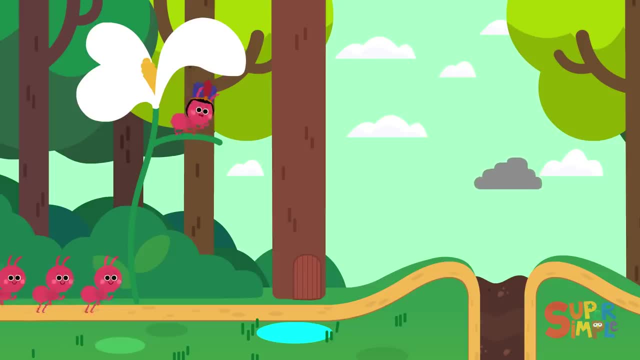 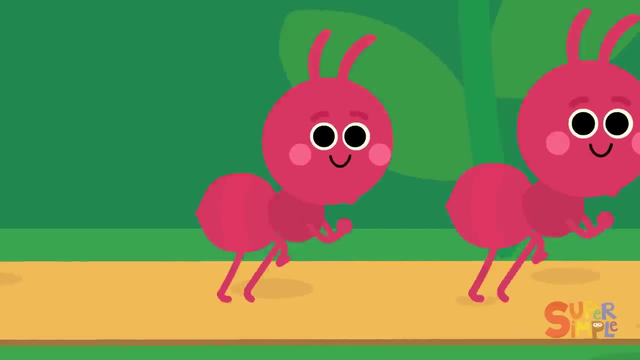 Boom, boom, boom. the ants go marching seven by seven. Hurrah, hurrah, the ants go marching seven by seven. Hurrah, hurrah, the ants go marching seven by seven. The little one stops to pray to heaven. 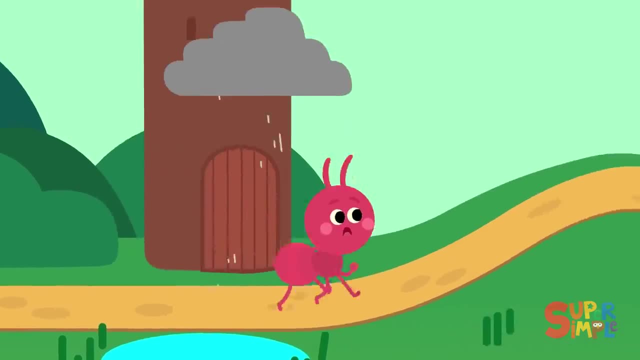 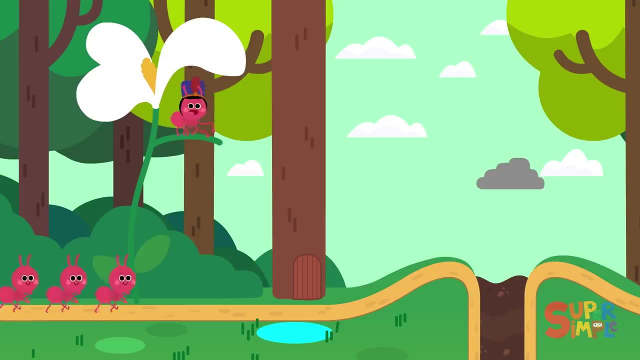 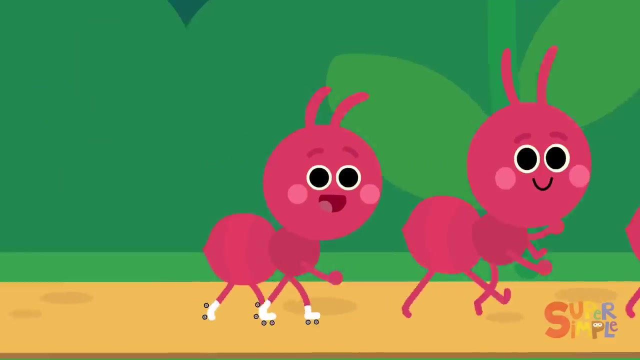 And they all go marching down to the ground to get out of the rain. Boom, boom, boom. the ants go marching eight by eight. Hurrah, hurrah, the ants go marching eight by eight. Hurrah, hurrah, the ants go marching eight by eight. 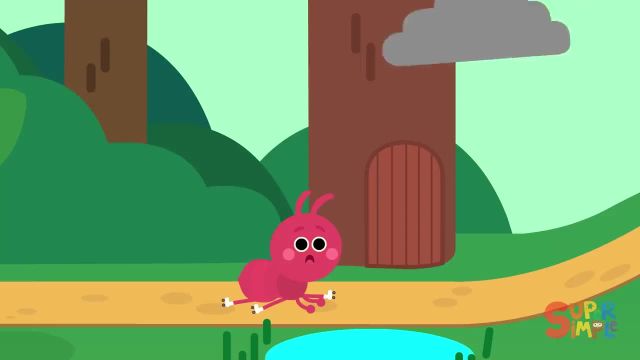 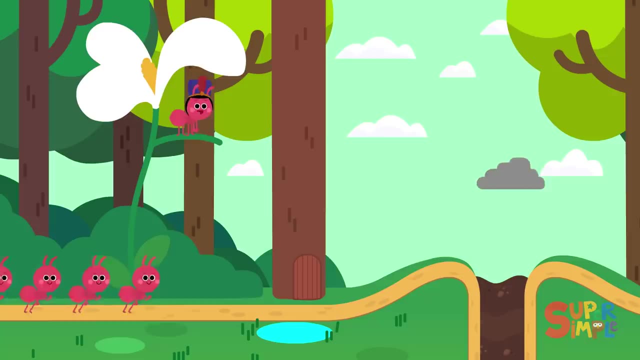 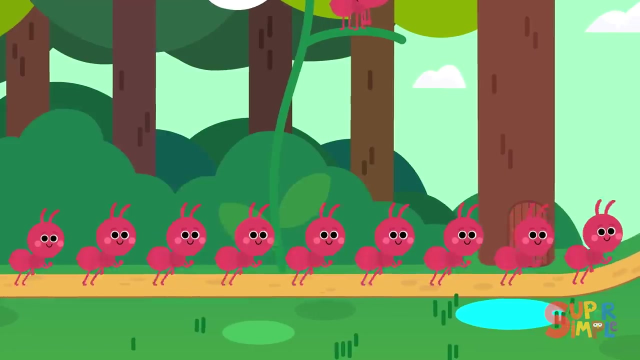 The little one stops to roller skate and they all go marching down to the ground to get out of the rain. Boom, boom, boom. the ants go marching seven by seven. The ants go marching nine by nine. Hurrah, hurrah, The ants go marching nine by nine. 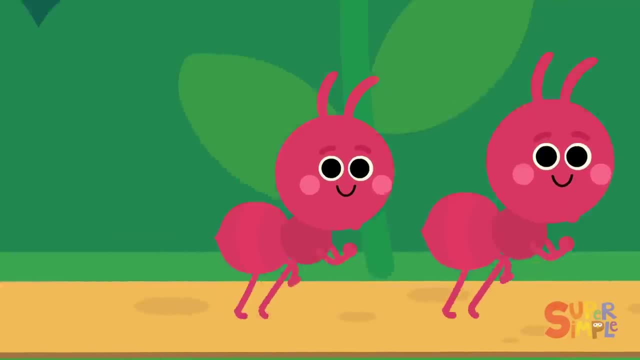 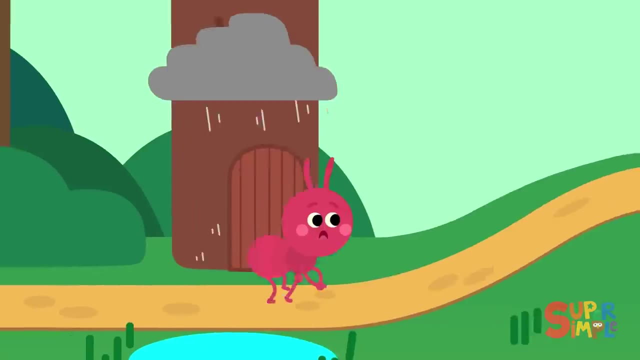 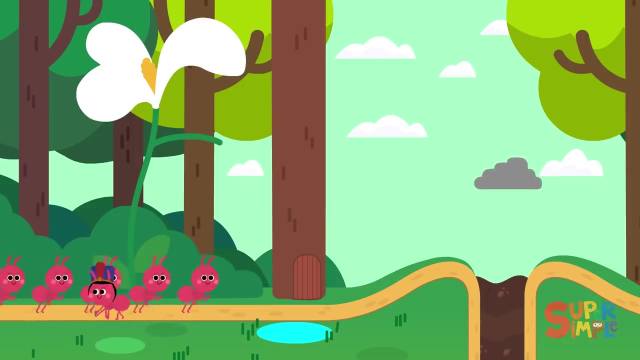 Hurrah, hurrah. The ants go marching nine by nine. The little one stops to check the time And they all go marching down to the ground To get out of the rain. Boom, boom, boom. The ants go marching ten by ten. Hurrah, hurrah. 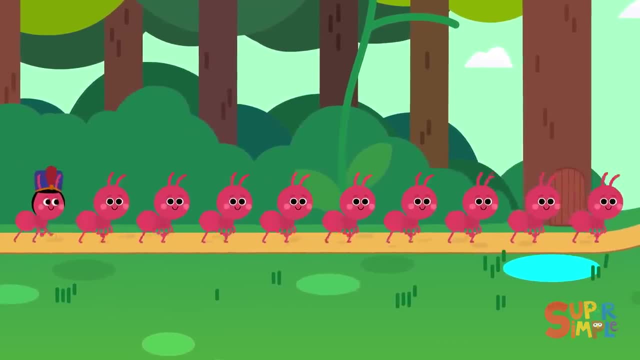 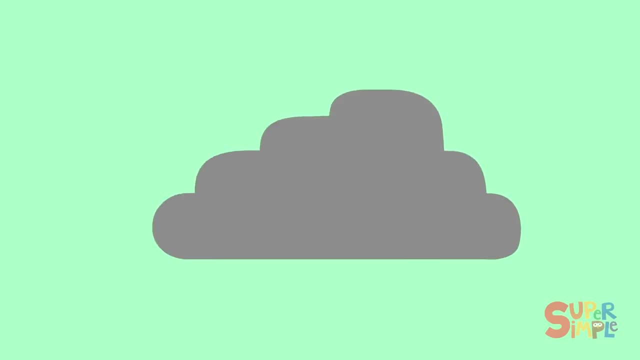 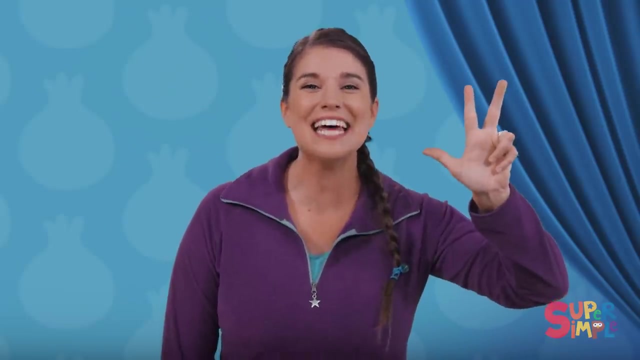 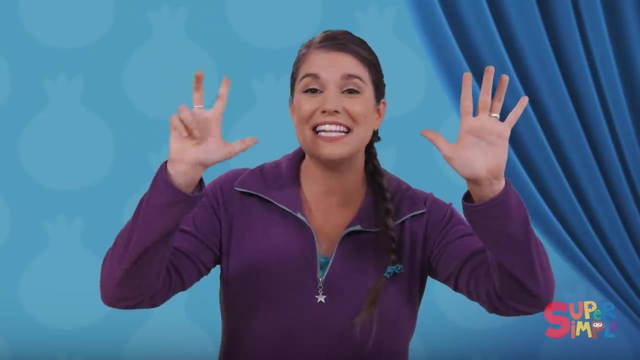 The ants go marching ten by ten, Hurrah, hurrah. The ants go marching ten by ten. The little one stops to shout the end: Hit it Katie. One little, two little, three little fingers. Four little, five little, six little fingers. Seven little, eight little.